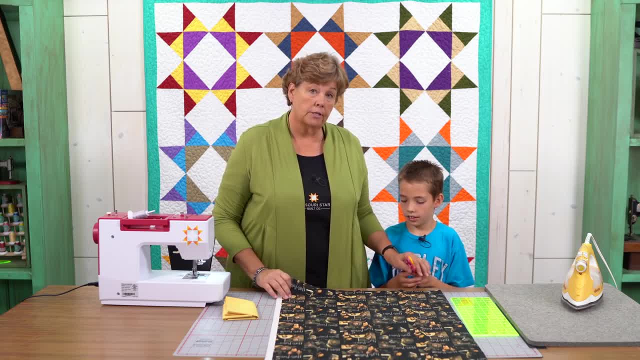 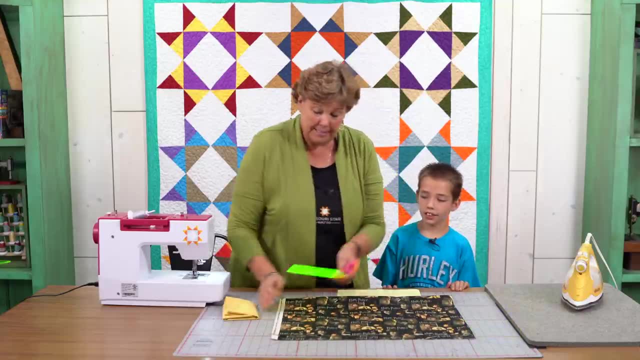 we're going to go ahead and cut off this little selvedge edge. Now, Talon is not going to be doing the cutting, I'm not ready for that yet, But I'll cut this for you. But Talon is sure going to sew it. So I'm just going to cut off this little edge right here. 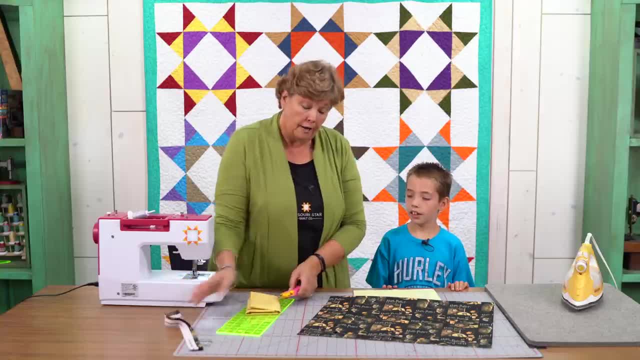 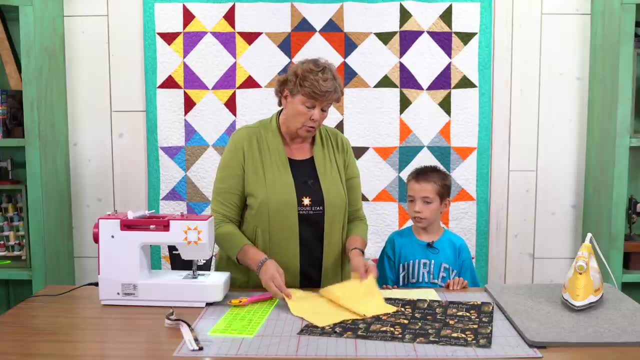 And slide right down there. Alright, Now for your cuff on your pillowcase- and this is just for a standard bed pillow, a twin size bed pillow. You're going to need nine inches or three quarters of a yard, And he's going to need a little bit of fabric And he's 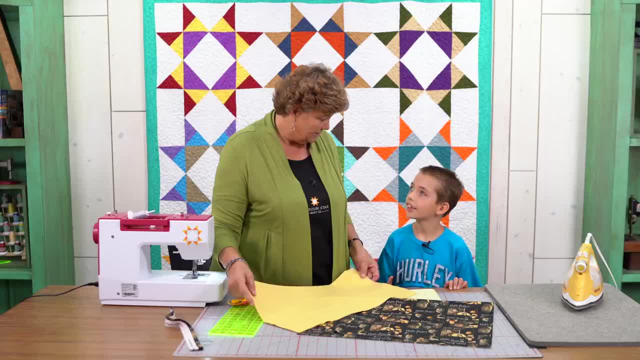 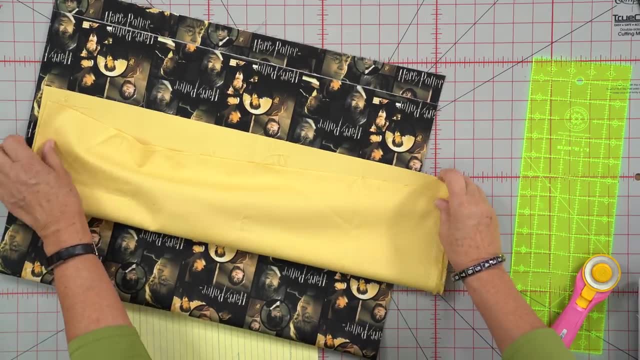 going to need a little bit of fabric, And he chose this cool yellow to go with that. That's kind of fun. Alright, now we do need to cut off our. we want to make sure this is the same size as our other piece, So I'm going to lay this on here like this, And then 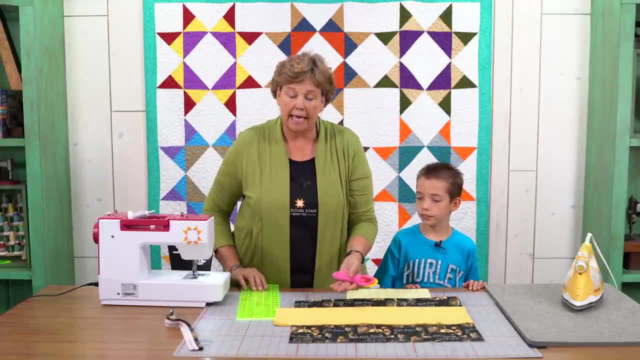 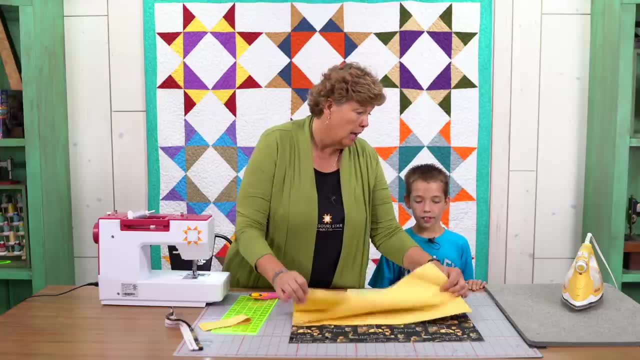 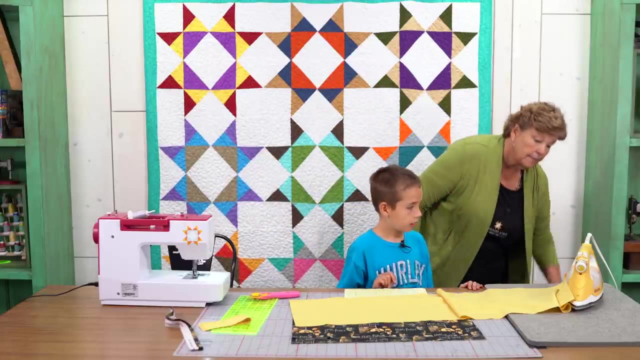 I'm just going to trim this edge off, so it's exactly the same size right here. Alright, Now what we're going to do is we're going to iron this in half. So we're going to come over here to the iron and I'm just going to move this little stool back here. 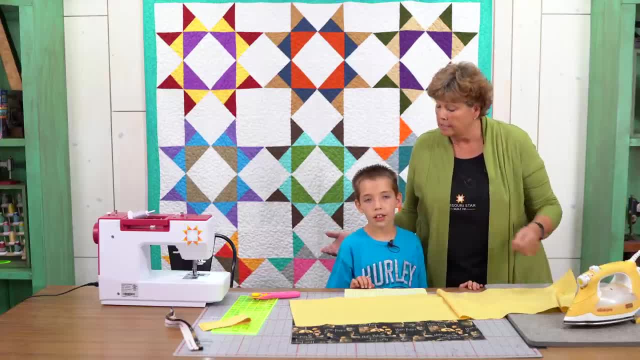 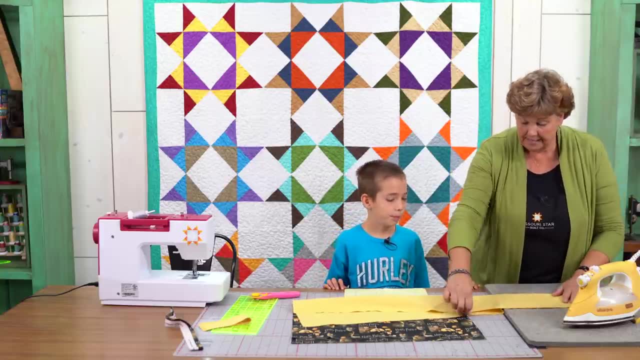 We brought Talon a little stooling to stand on, and he informed us he was tall enough. He did not need that stool. So he's grown from last year too. Alright, Talon, can you iron? Um, I don't know how yet. 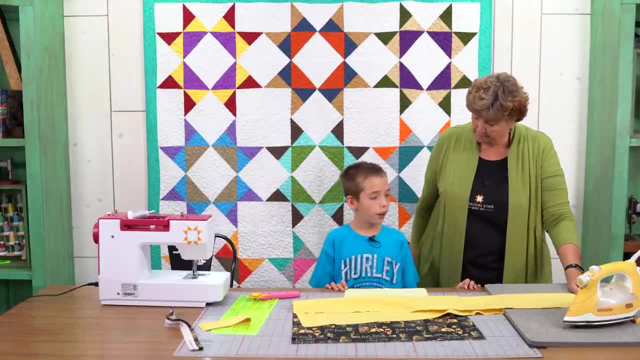 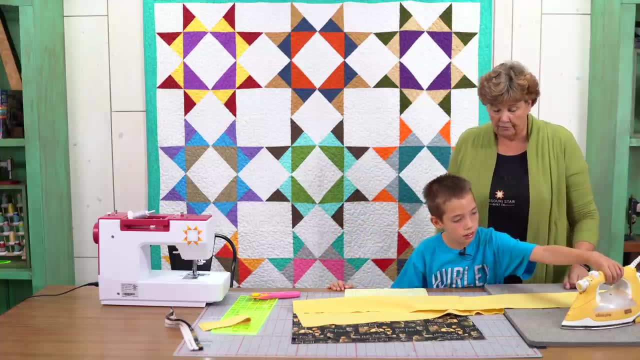 Alright, But I'm hoping I will. Well, we have kind of a magic iron right here. Touch, touch this iron right here, Take a hold of the handle And the feet go down. Isn't that cool? So what we're going to? 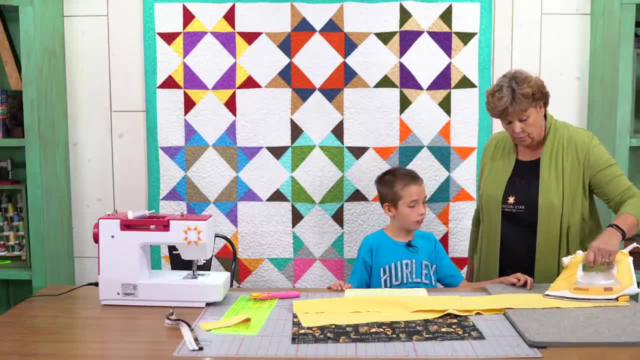 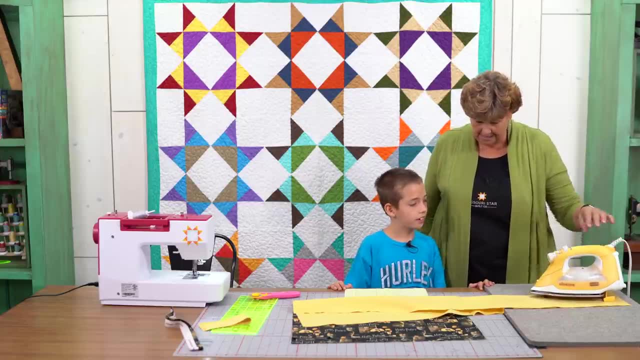 do is we're going to touch this and we're just going to put it right on this edge, right here Now. the nice thing about this iron is that when you let go, it lifts right up. Isn't that cool? So I'll slide this over and I'll let you do this next part right here. So we're. 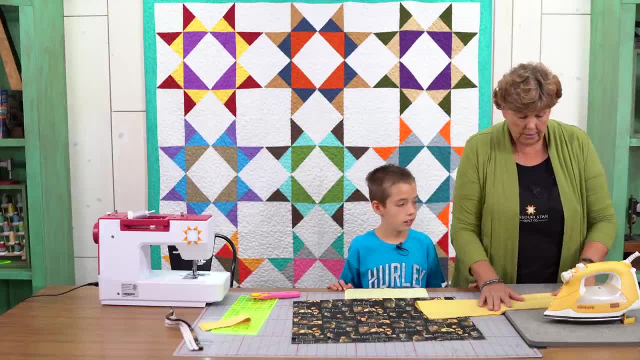 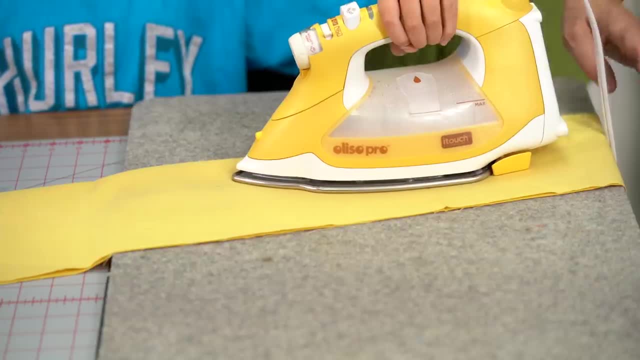 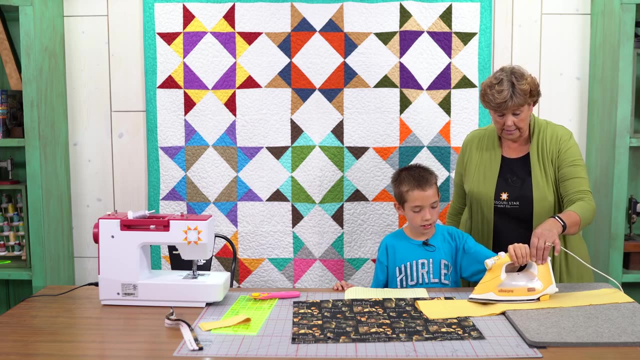 folding this so that the edges are even Just like that. Go ahead, you grab that iron Now, lift it over here And iron that down. We want to make it nice and flat. There you go. Now let's come back here a little bit and catch this edge right here. You did a good job right there, Look. 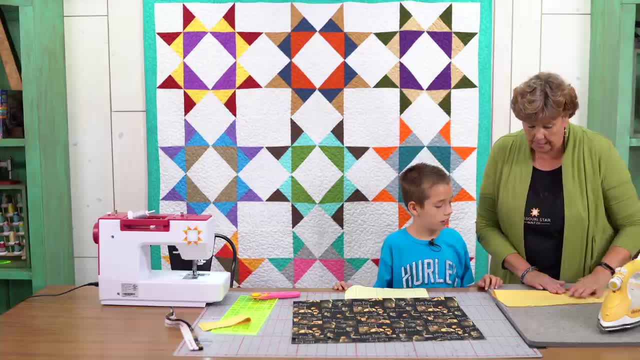 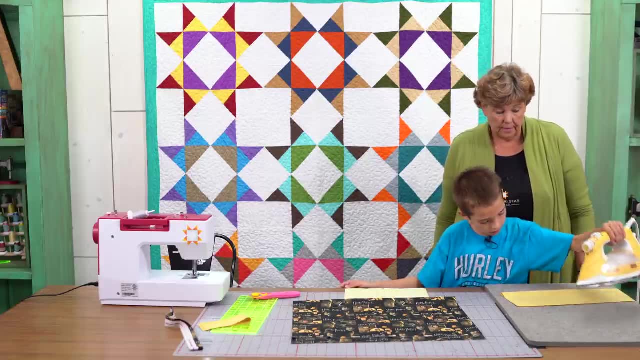 how crispy that is. See how nice, see what kind of crease that makes. That just means our fabric is not going to go anywhere and it's going to lay a lot nicer. Alright, go ahead and grab that iron. Oh look, he's getting brave. You're doing good, buddy. 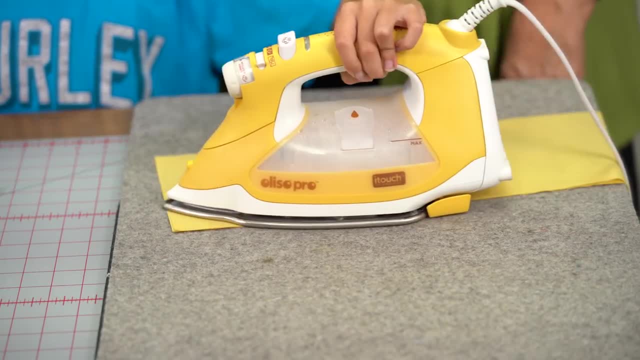 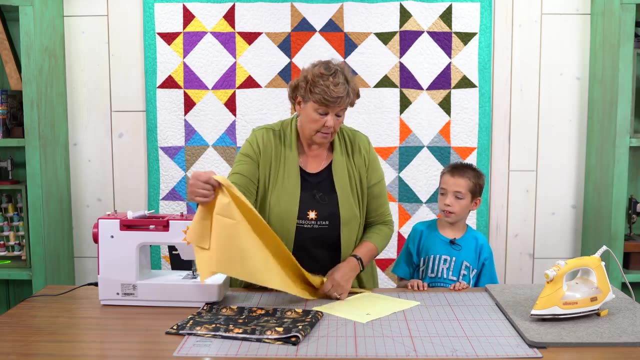 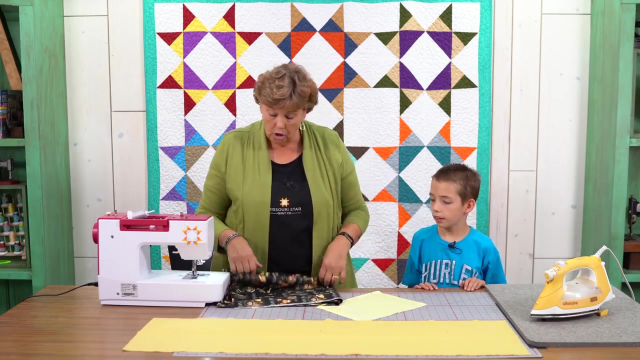 Alright, that is a good job. You are doing a good job ironing. Alright, now it's time to put this together And we're going to open this up, but keep our right side to the top, So we know this is the right side, because that's the fold. Then we're also going 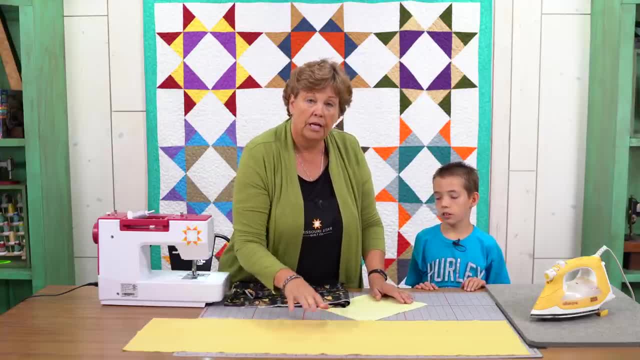 to, and I don't know if I I might have said this wrong before. This is ¼ yard of fabric, nine inches, And this big piece is ¾ yard of fabric And it is 27 inches. Alright, let it rest. Now we're going to fold this over here. Now let's go back to this side. 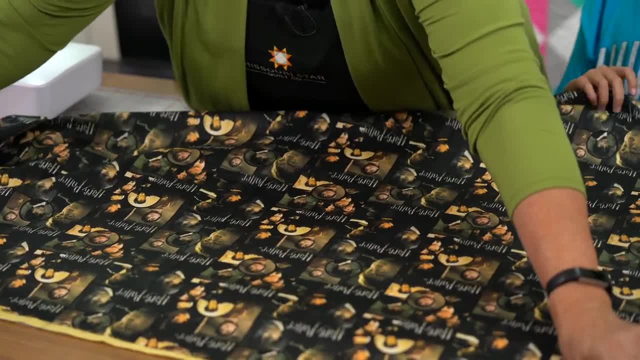 Grab your stitch marker Text on the screen. Okay, so this is how we're going to fold this over. So we're going to fold this over to the bottom, like so, And then follow them onto the outermost. Alright, so again, this is. this goes right up to the top edge, like this And everything. 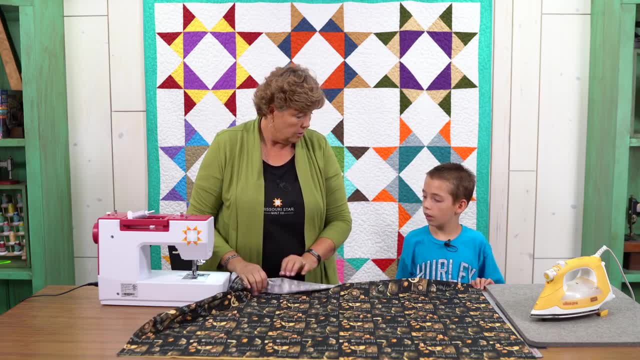 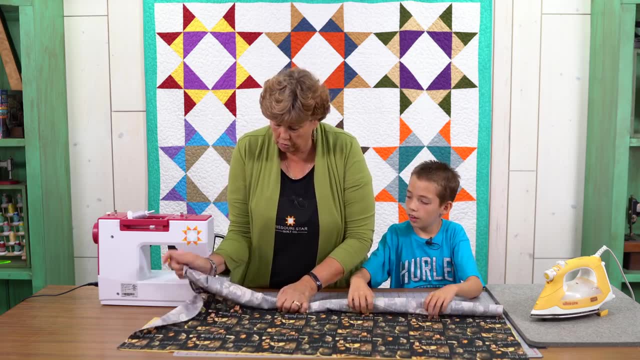 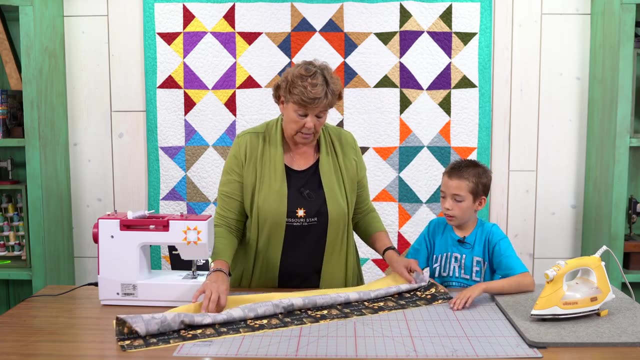 facing upward, And then we're going to roll. So you help me roll. We're going to roll up here like this: Rolling, rolling, rolling. Keep those doggies rolling, Alright, stop. Now we have to bring this close to us, because what we're going to do, let me move this. 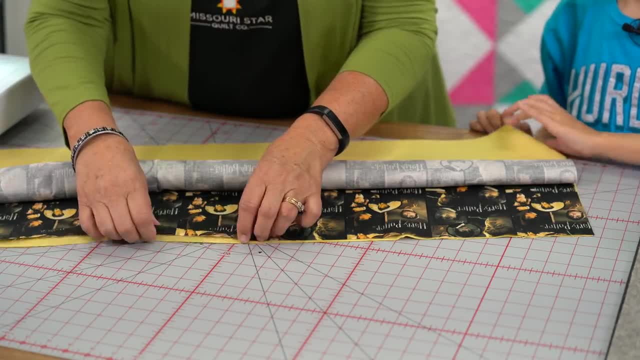 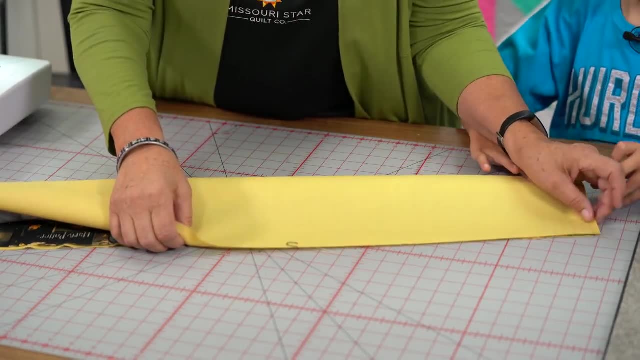 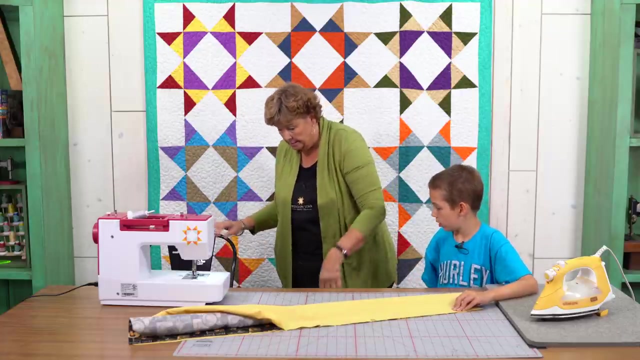 paper. What we're going to do is we are going to make sure all these edges line up exactly, And then we're going to fold this over and pin this, but not catch our fabric in there. So we need some pins. Let me see if I can grab some pins real quick. Here they. 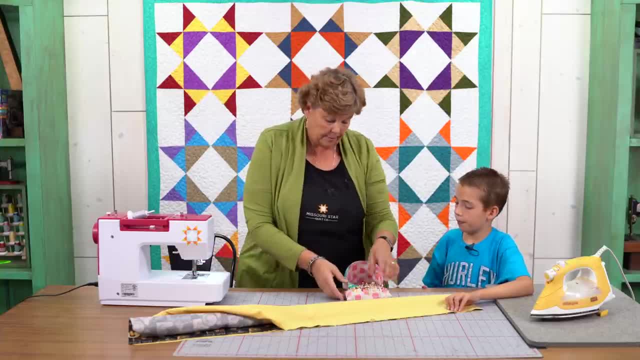 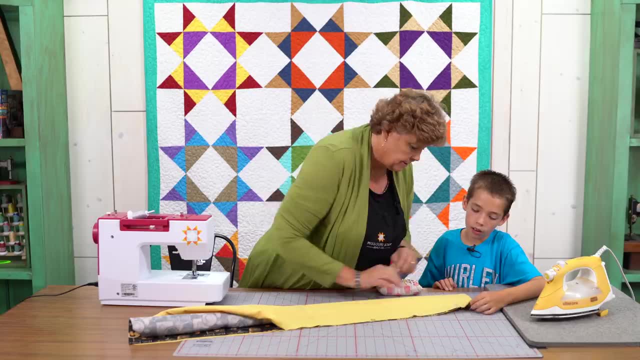 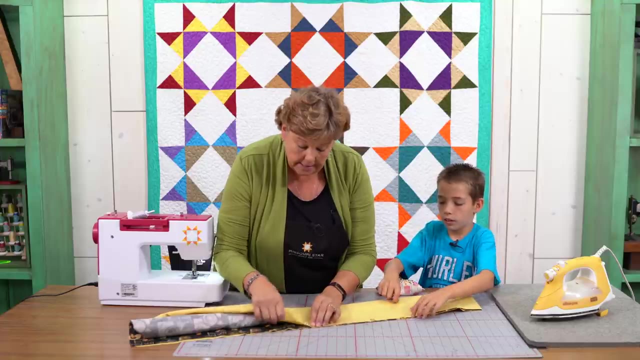 are, Alrighty, here's my pins, And so what we want to do is we want to put a pin in, We want to stick it in there and do that. Alright, Ok, Can you do that? Uh huh, Alright, I'll start over here on this side, And your pieces are lined up exactly. 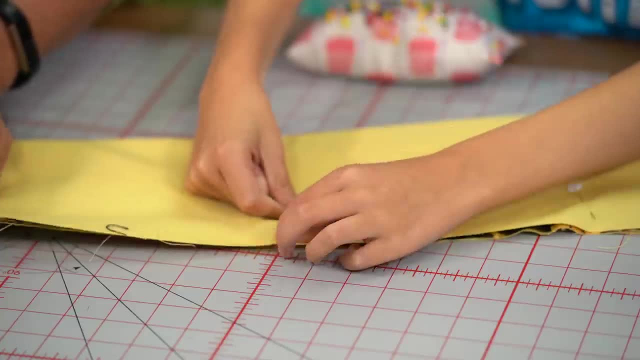 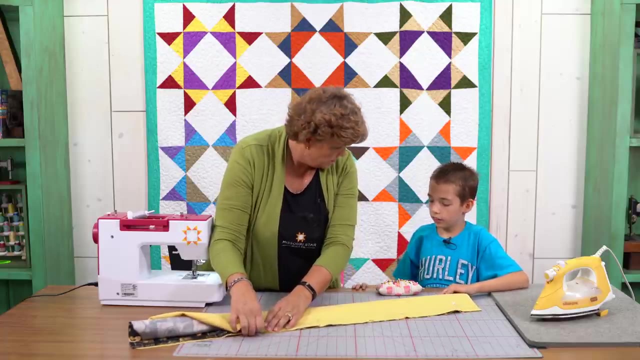 What's your favorite part about Harry Potter? Um, I like that. it's a magic school. Oh yeah, Would you like to go to a school like Hogwarts? Uh huh, You would. That would be fun, wouldn't it? It would. 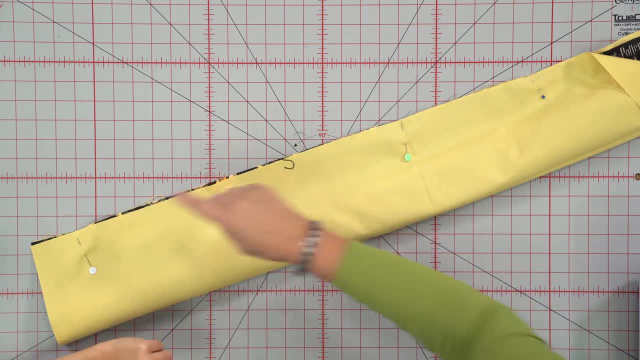 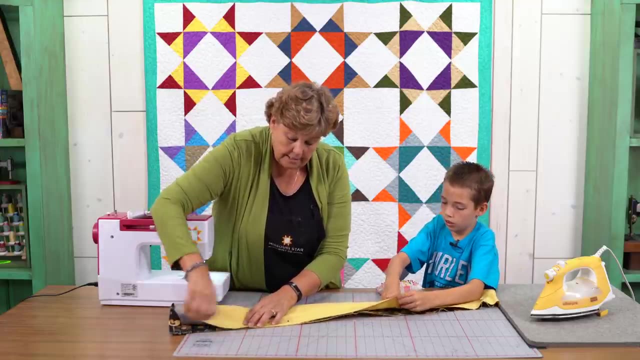 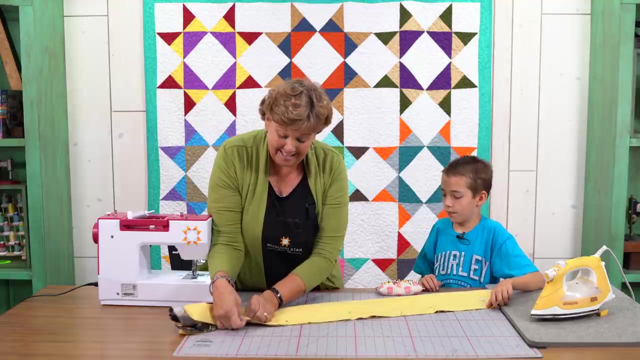 I bet: Alright, let's put two more in here. We don't need a ton, but we need it to stay right together. This is actually kind of. this pillowcase has so many names. Lots of grandmas make their kids pillowcases with this, with this pattern, And it's they call it a burrito pillowcase. 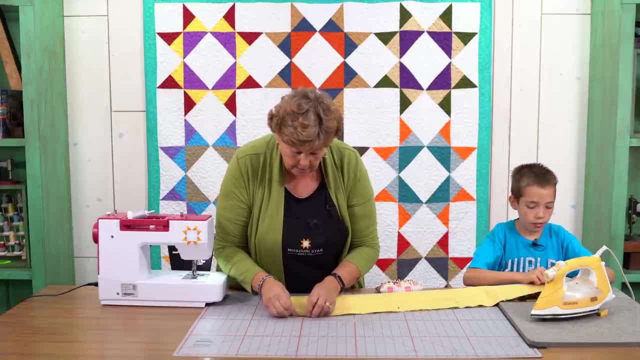 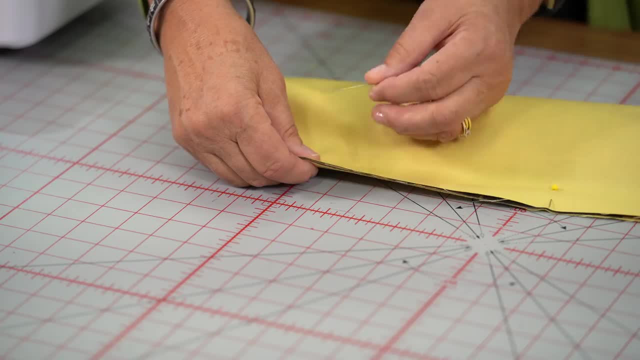 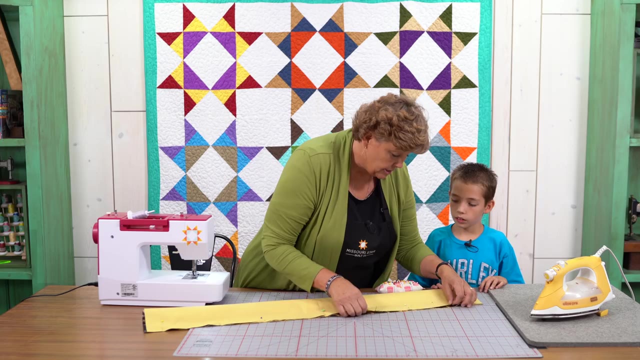 and a sausage pillowcase, All kinds of names. Alright, I'm going to pin this one. Look at you pinning all on your own. Good job, buddy. Alright, Alright, let me make sure. Oh, ok, now see right here. This has to get all the layers. We have to get all the layers. So 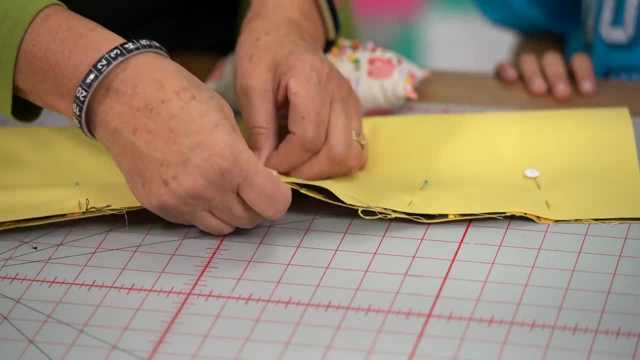 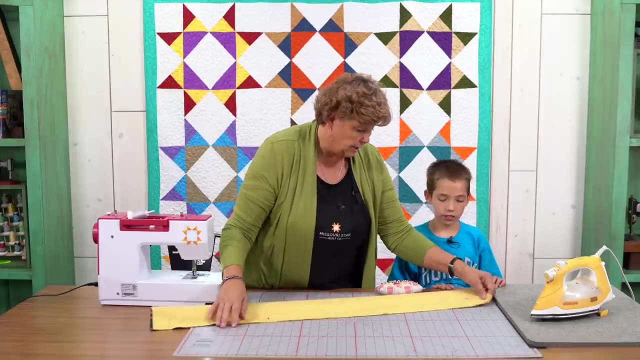 we're going to stick this through all the layers. We don't want any of those to slide. So your pinning work was fabulous. We just have to catch them all, Alright. Now what we're going to do is we're going to take this to the sewing machine And you can come. 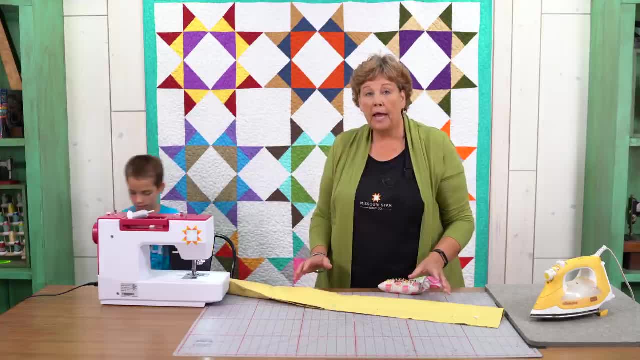 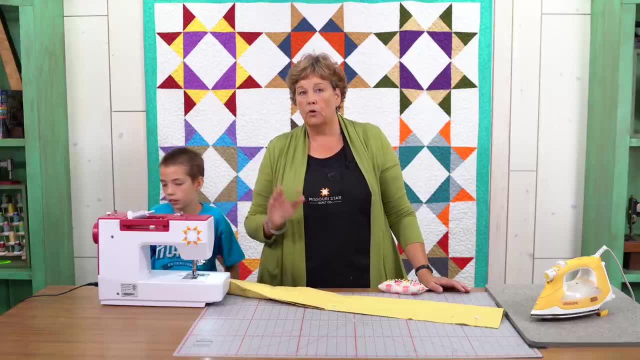 over and get settled on your sewing machine. Talyn practiced on his paper so he can stay on the line, so I know that he can. Our sewing machine also has a speed control. I'm going to slow it down a little bit so that it doesn't race off when you take it. He's up here. 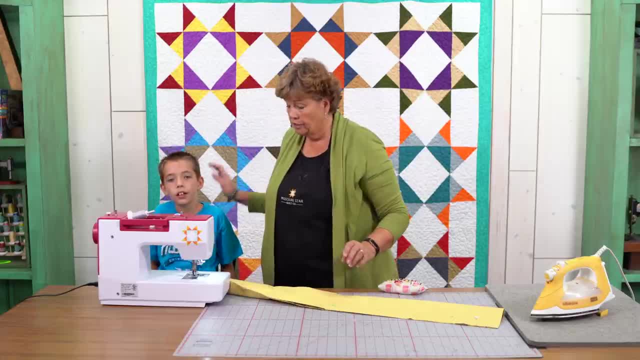 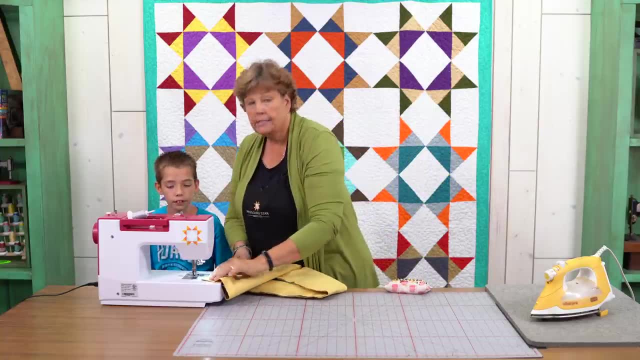 on my high chair, But there's a pedal down there and he can reach that pedal perfectly, And we are just going to sew right along this edge And it doesn't matter if it's a quarter inch or a half an inch, It matters that it's the same. So what I'm going? 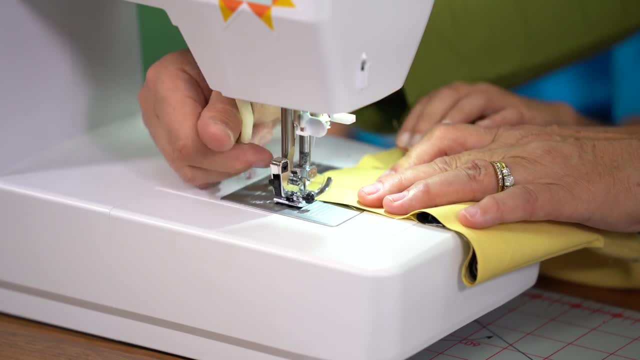 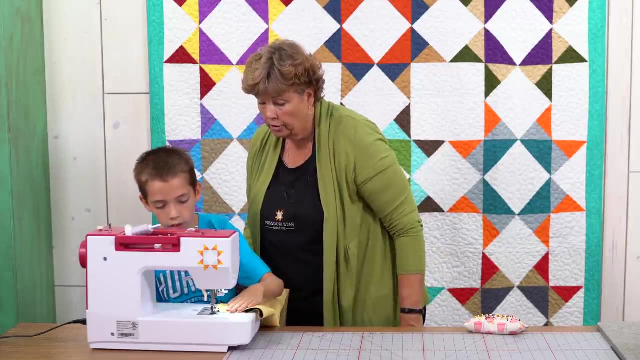 to do is I'm going to line this fabric right up along that edge, ok, Just like that. And then I'm going to kind of hold this And help you feed that through, And you're going to push the motor, Put your other hand. 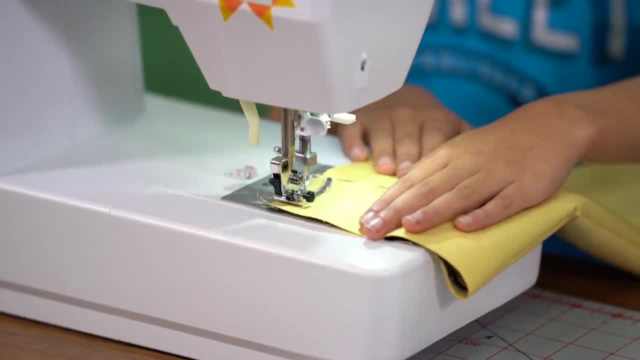 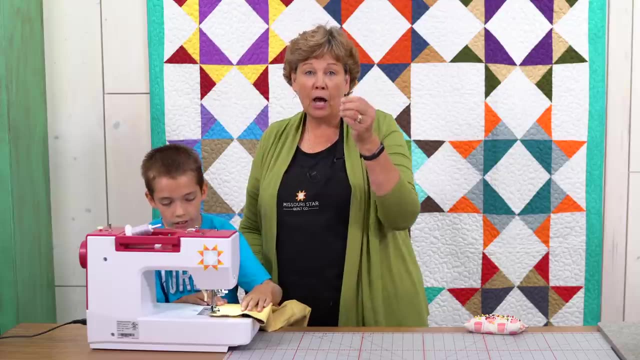 up there and help hold that fabric, And we're just going to sew. We're going to sew this whole long thing. Oh, you know what? You are so smart. He took the pin out before he even got there. Yeah, you don't want to sew off a pin. What can happen if you sew over a pin? 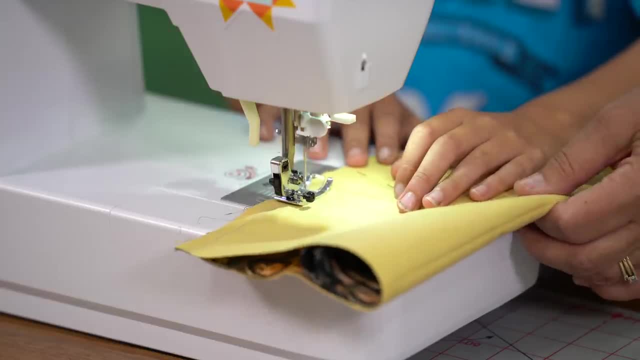 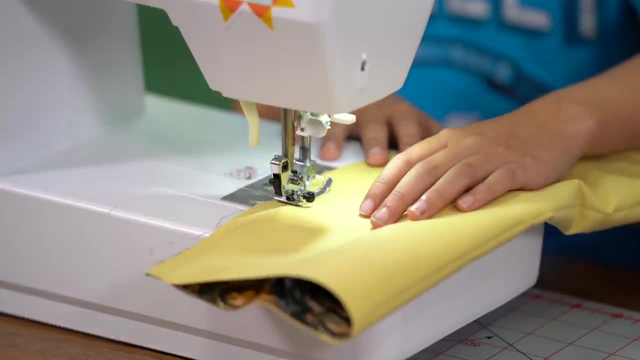 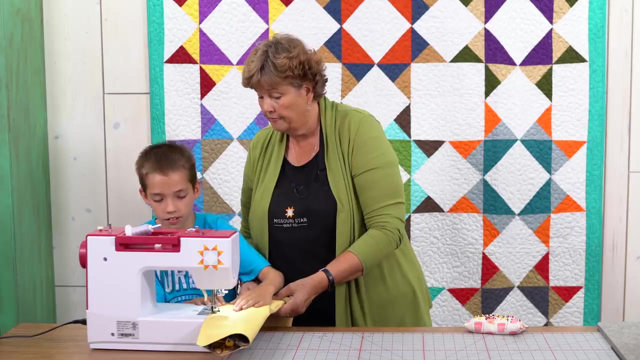 It, it will break. It could break the needle, couldn't it? Uh huh? And that needle could do all kinds of crazy things. Good to be safe, There we go. You think you could go a little bit faster, Uh huh. 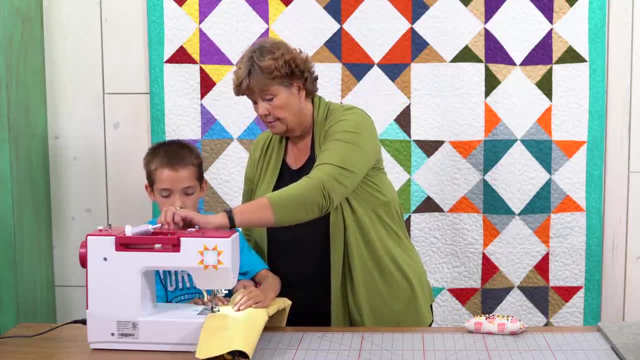 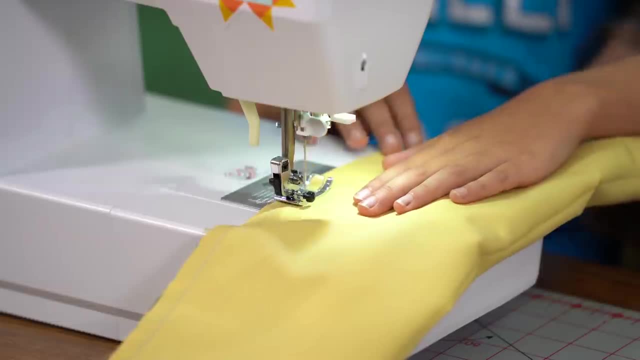 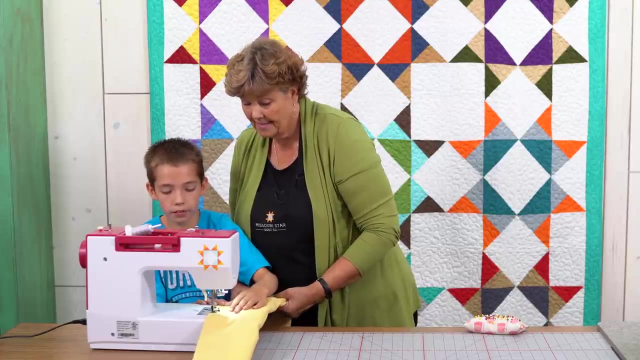 Alright, I'm going to turn it up just a little bit. Alright, now, slow, there you go. Perfect. So what's your favorite part when you come to Missouri? Um, I like that most of my family is here. Yeah, you've got lots of family here, don't you? 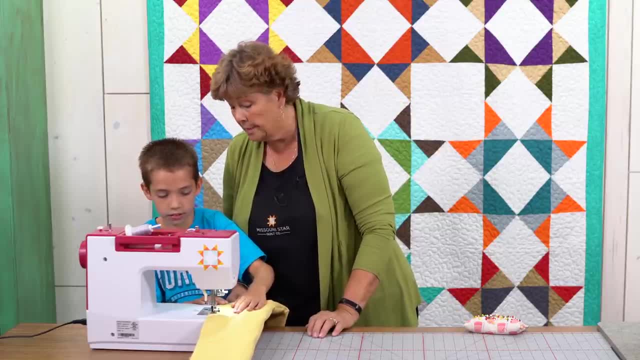 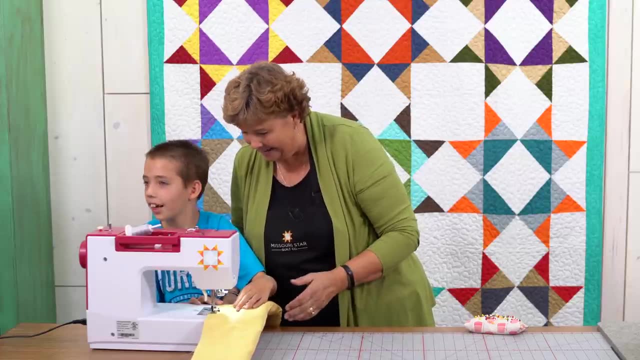 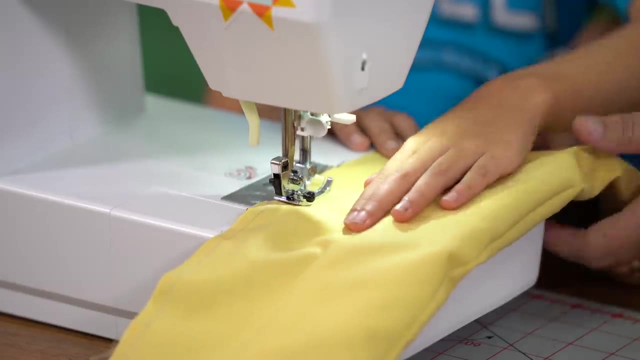 Yeah, Uh, huh. And who's your favorite family person? Grandma, Grandma. Good answer. Wait, what about your dad And my dad? Oh and my dad, Oh. good answer. He knows how to play those cards, right Alright. 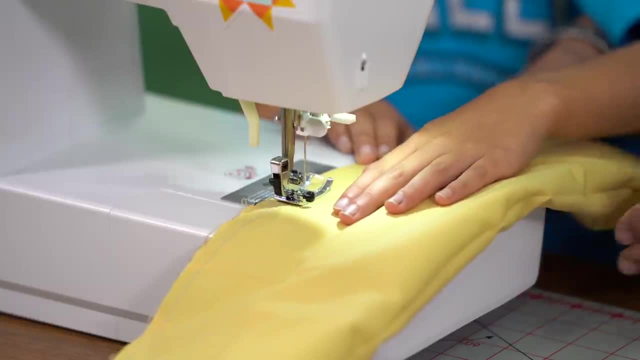 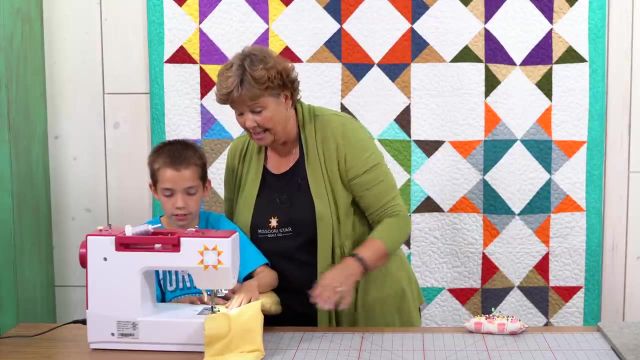 we're staying right along that edge. You're doing so good, buddy Gosh, you're so good. You're doing so good. Yeah, Thank you so much Last year. the last time I sewed with Talyn was last year, and uh. 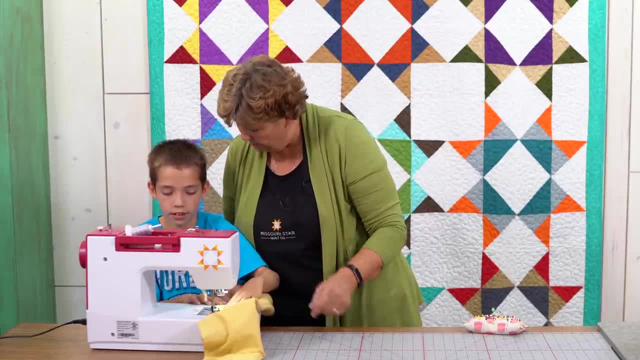 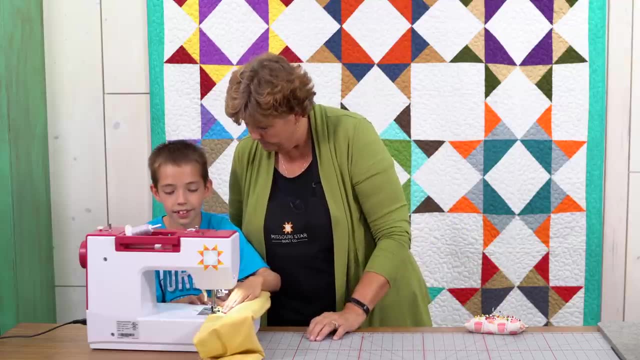 he had to actually sit on my lap last year, and now you're in the chair. all by yourself, We might even be able to turn him into a quilter. What do you think? Uh huh, Yeah, You want to learn how to make a quilt. 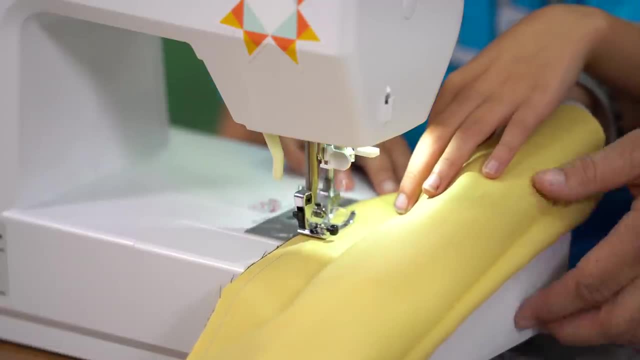 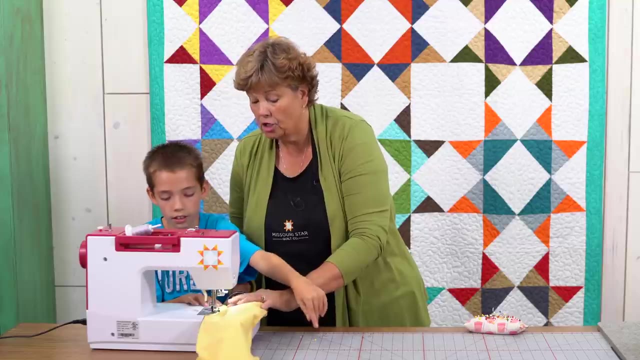 Uh huh, There are a lot of men sewers out there. you know Your dad is one of them. He has a quilt. Do you remember the name of his quilt? No, Uh, it's called Josh's Seed. It's called Josh's Star. We'll put a link for that below too, so you can go see. 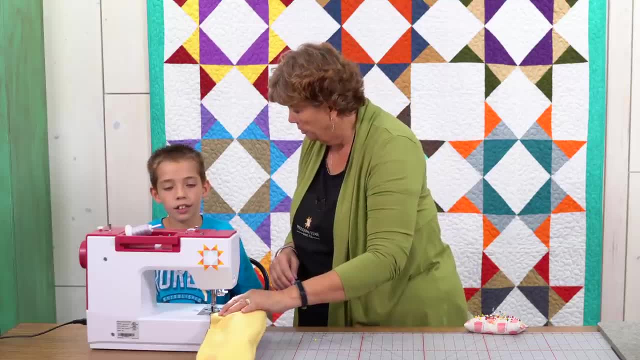 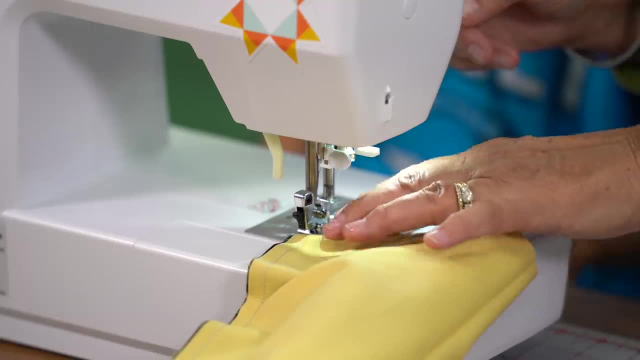 it. He also actually made up another one called the Blipper. He didn't film that with me, but he. that was his idea. Alright, now on your sewing machine, this is a backup button, so I'm going to push the backup because we want to. we want to make sure that it. 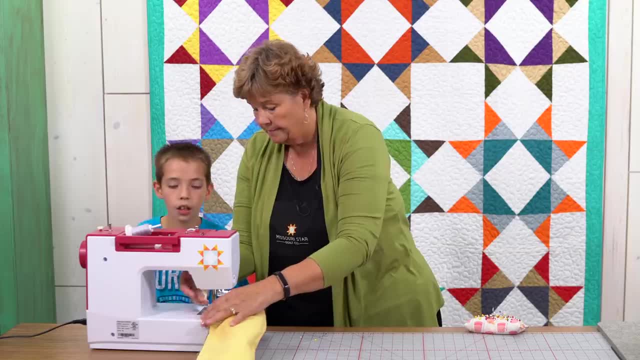 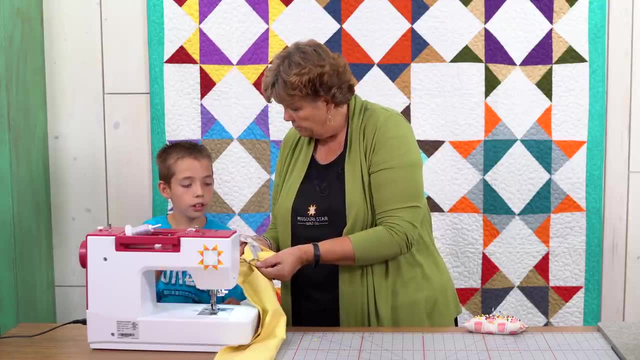 um, it sews There, we go. Alright, Now we're going to clip this thread right here, And then what I want you to do is see: all the fabric is inside there. Uh huh, I need you to pull that out. Can you pull that all out of there? 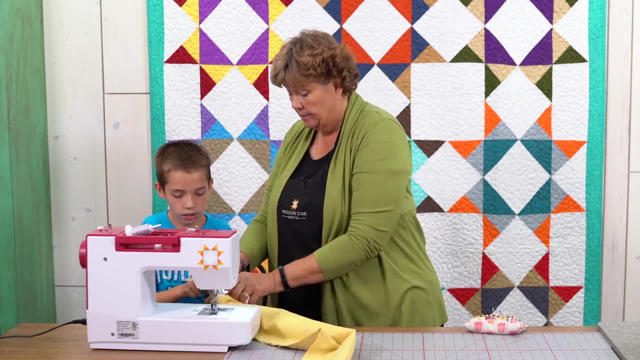 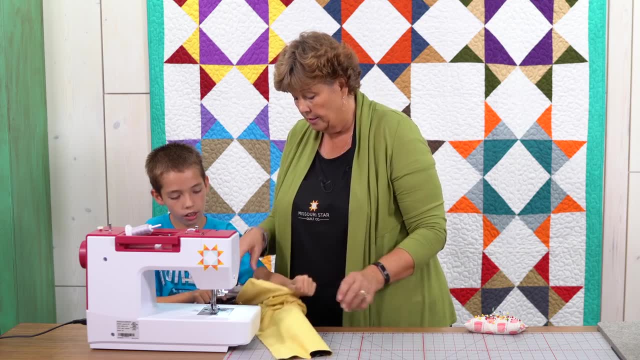 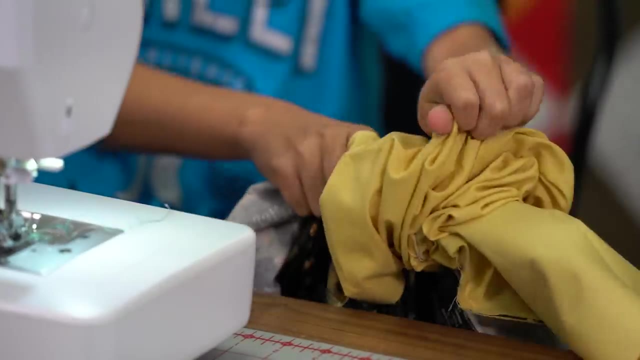 Yeah, It can only come out one end. Two people can't really help with this. You just got to pull it like this: Get a hold of that roll. See, right here on this front. part is there, you go, You got it, You're doing it. bud, You're doing it. The nice part about 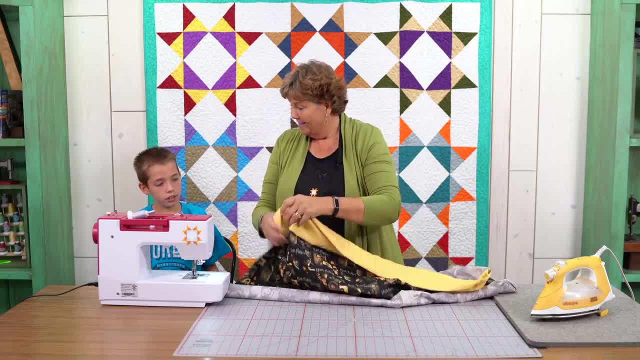 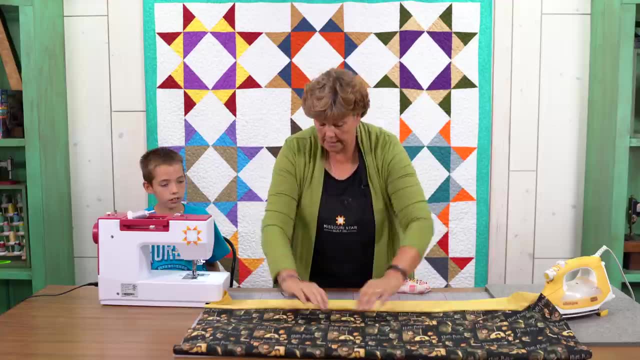 this. alright, now see right here, Look at this, Here it comes, Here it comes, Here it comes. So the nice part about doing it this way is: first, we've already ironed that nice fold down there, so it's going to lay down really nice And there are no seams. that 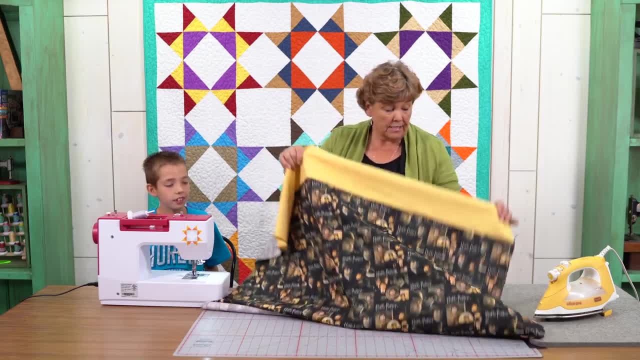 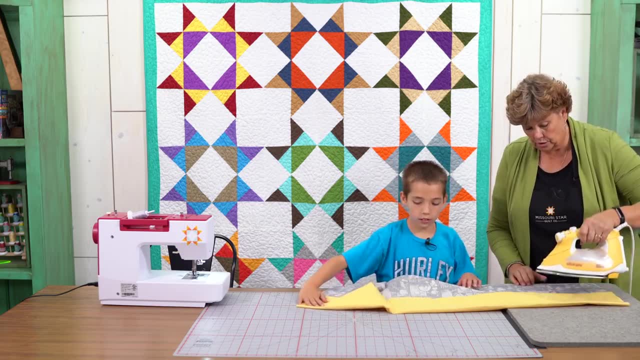 show on either side. Isn't that cool, Uh huh. So let's iron this again. And we're going to iron where we sewed the seams, So we're going to kind of push this up like this with our iron. So we're just going. 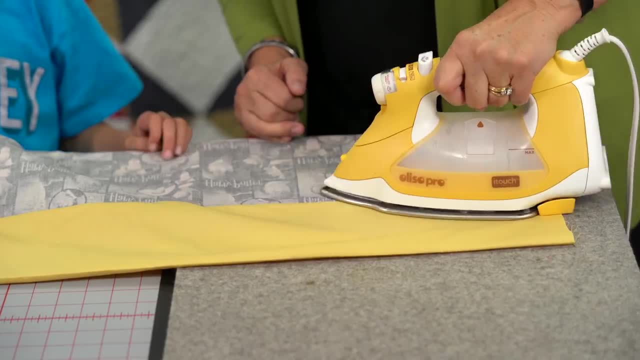 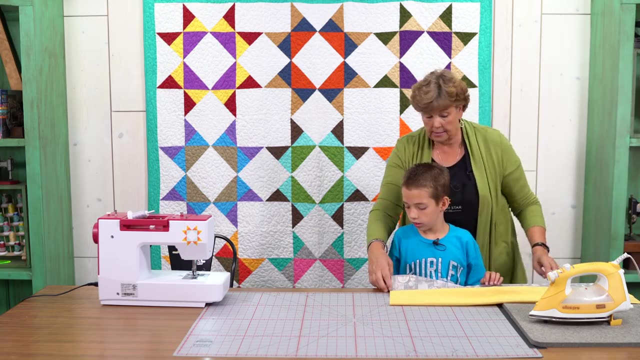 to go up like this, And we'll do this on both sides, So we don't have to go all the way to the top. Just a little bit along there. So there you go. Okay, Just a little bit along there. So let me slide this over. Let's move our pins, You. 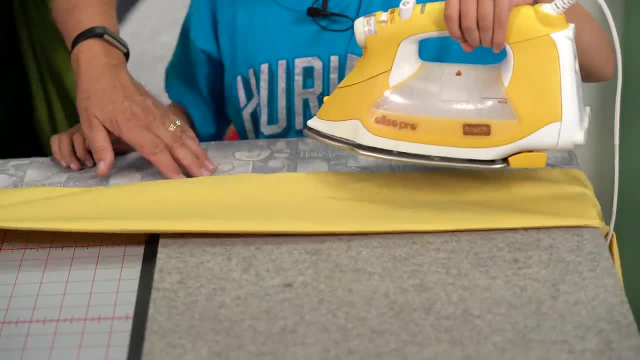 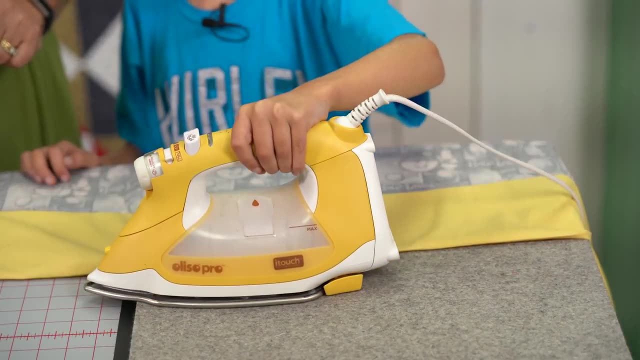 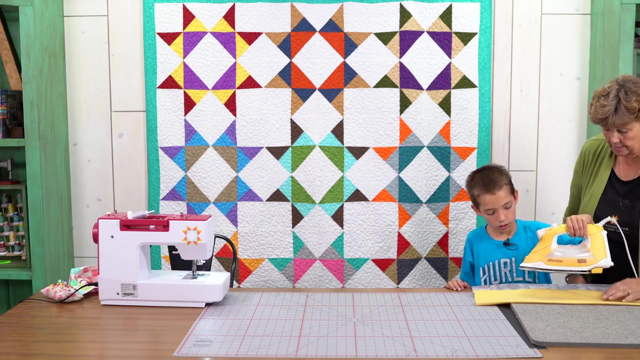 go ahead and iron that part. So put it down here, no, put it on the fabric like this, on this pillow part, and then push it up like that, And that will make that part move away from that seam. Alrighty, Now over here one more. Let me scoot it. Lift it up There, you. 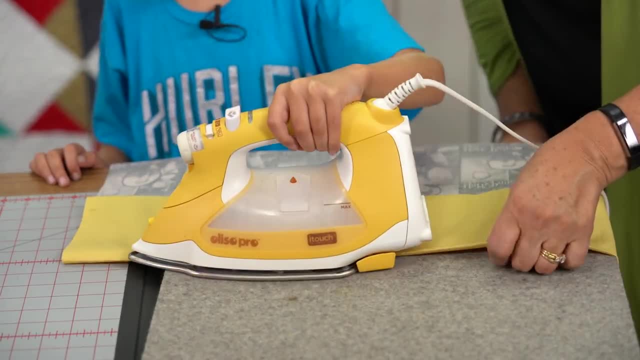 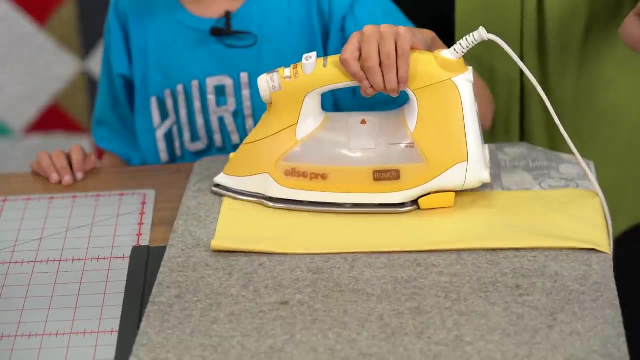 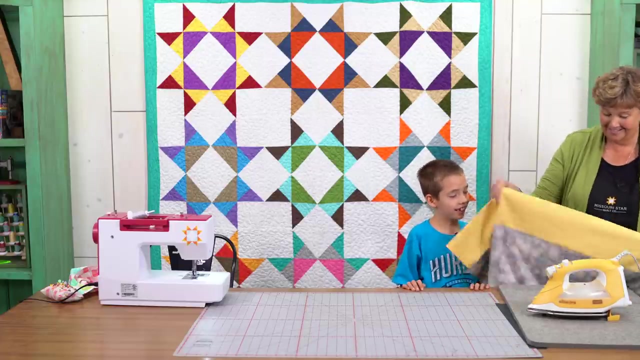 go One more. You got it, buddy, You're doing great. Alright, one more, Oop, hang on, Lift it up. There we go. Now we're going to do the other side. Alright, let go. There it goes. Isn't that a fun iron. 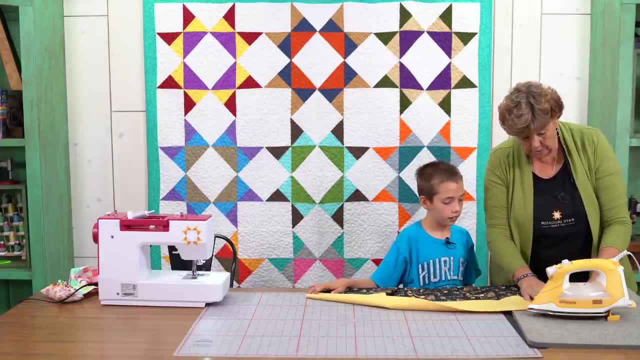 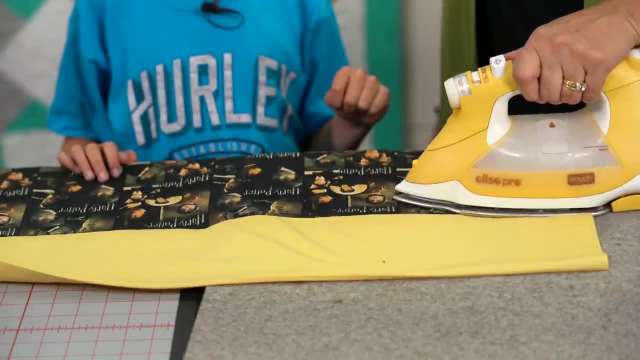 Uh huh. Alright, now see here, this has a little bit of a fold in it. We don't want that, So we're going to do the same thing. We're going to put it on Harry Potter's face: Push forward. We won't leave it there long enough to burn him, just to make him nice. 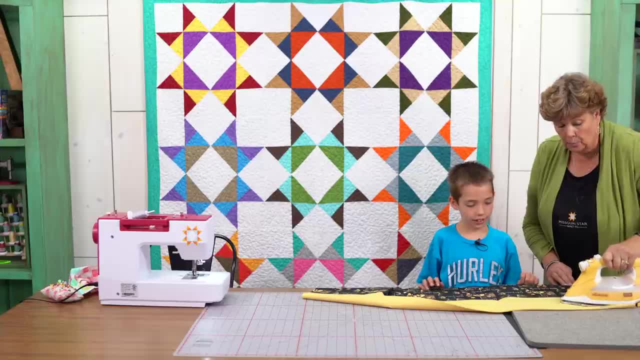 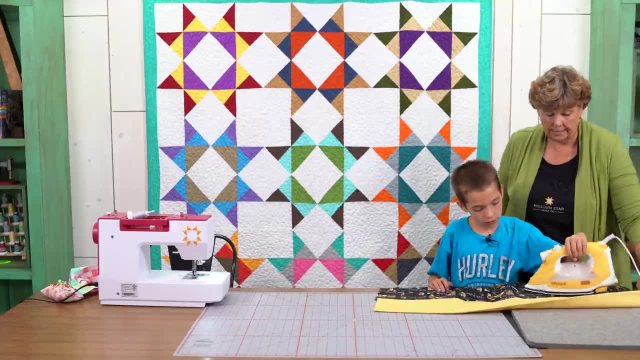 and creased. Alright, let me move this, And this time we want to go all the way to the edge. Okay, All right, here we go Ready, All right down on Yep and just push it up there. 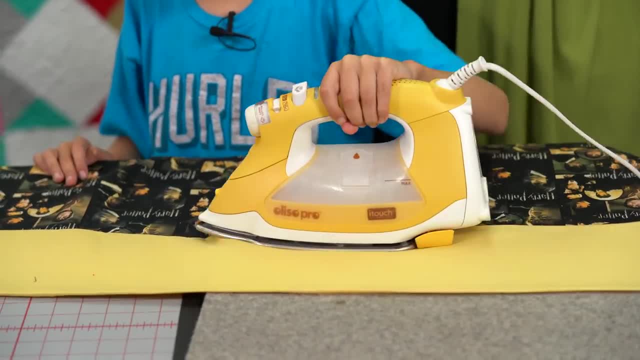 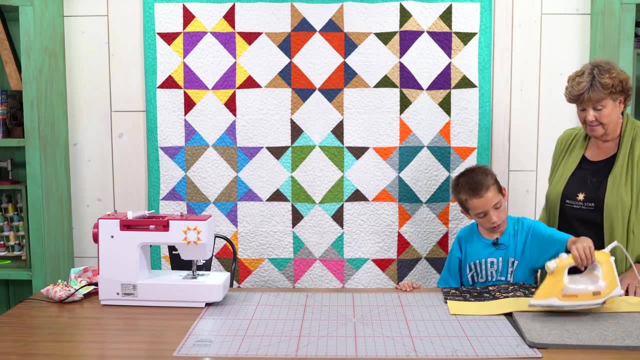 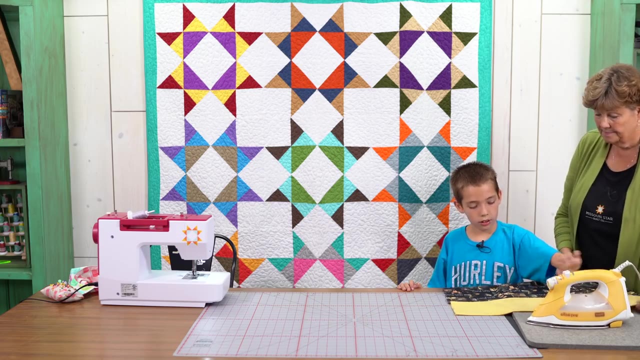 There you go, perfect. Uh-huh, Aw, you're doing great. Alright, let me slide this over a little more. Push it up, Awesome, And one more. Let me do that again. All right, There you are. 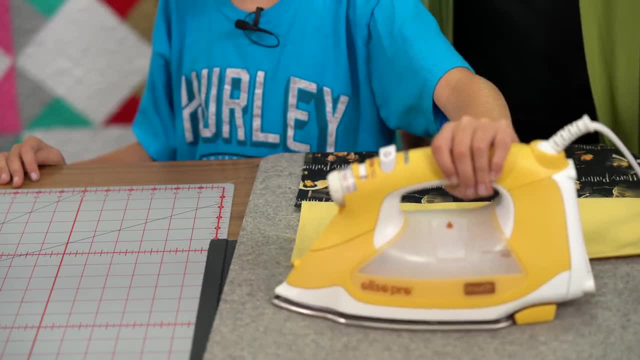 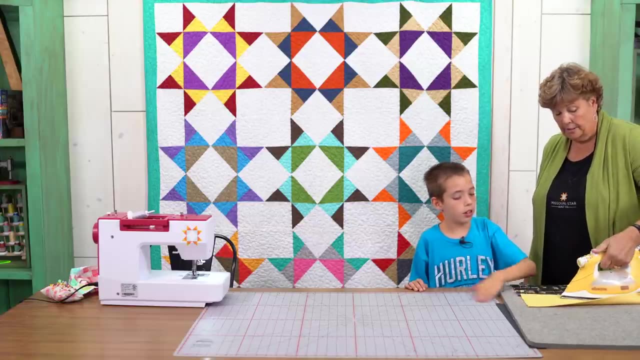 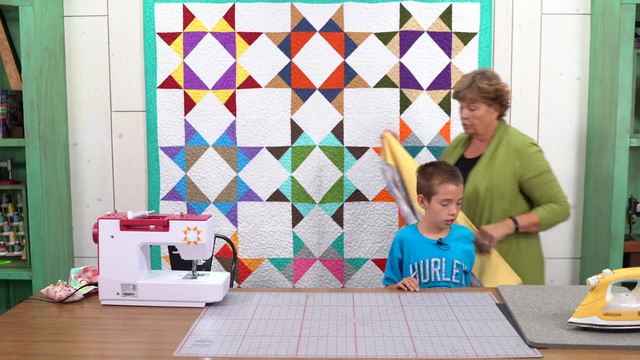 You got it. Alright, let me get. I'm going to put it right here and I'm going to do a shot of see if I have any steam in here. I don't have any steam in here, But I do like me a shot of steam, Alright, now what we're going to do is we have to sew this. 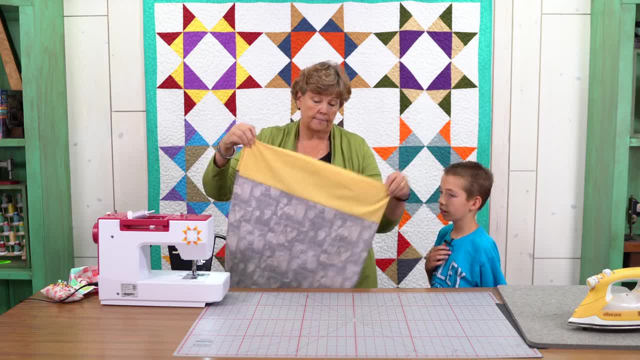 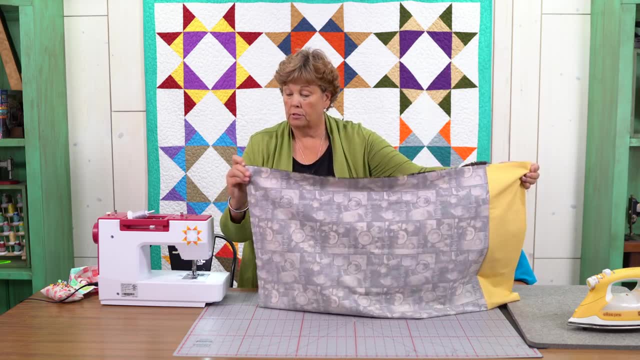 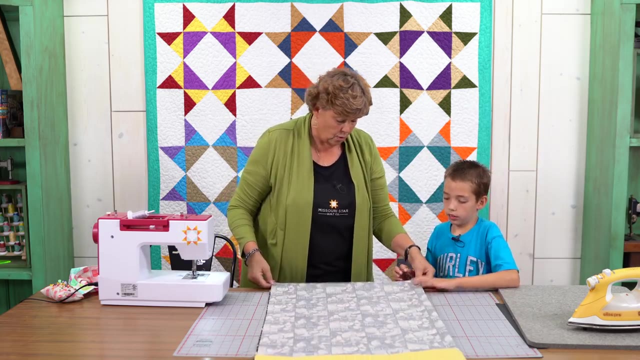 closed and make a pillowcase. So we fold it in half like this And we're just going to line these up and make sure that they match- And they should match pretty good- And then line this bottom up. So why don't we sew across this bottom first? Now you can pin. 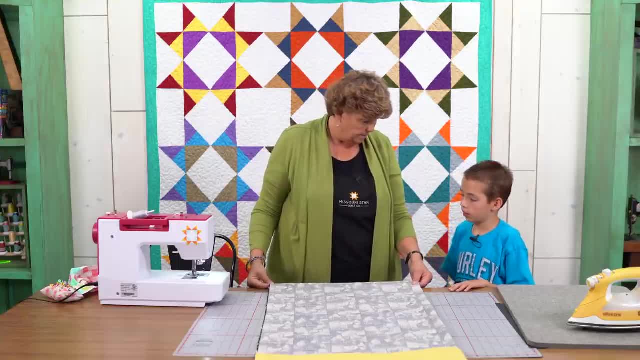 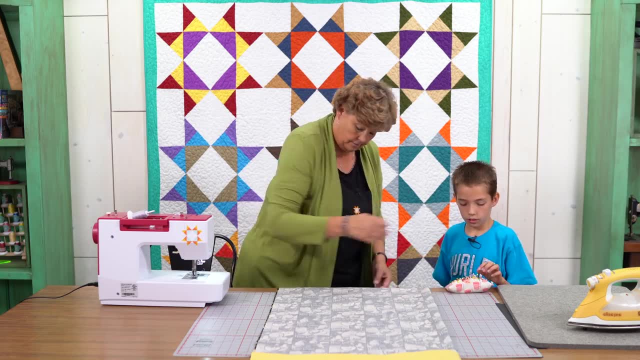 this, if you want. Do you want to pin it or do you feel comfortable without pinning? I think we should pin it. Ok, alright, let's do that. Let's just put a couple pins in there to make sure that it holds together. So I'll pin it right. 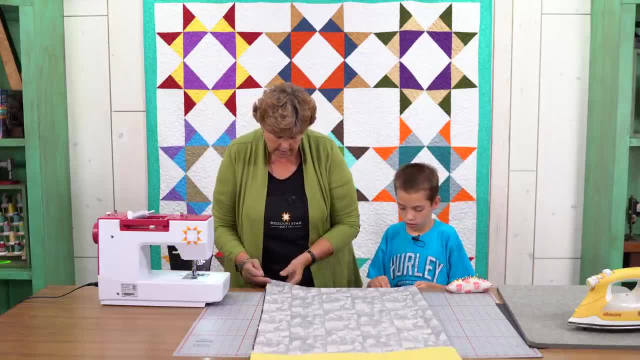 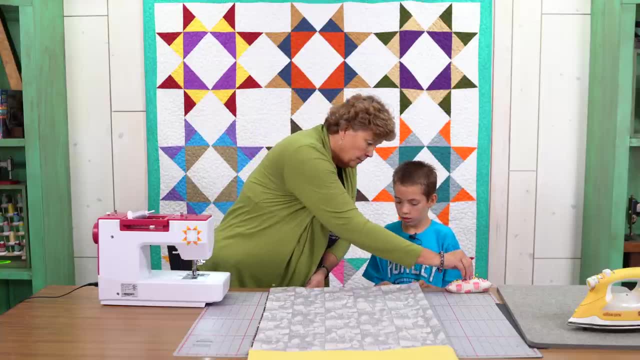 here. Ok, You know pinning is one of those things, Talyn, that's really personal. Some people like to pin And you always want to pin. so your pin comes out to the edge, your pin point comes out like this: So you stick it in and put it through there like that: But pinning- 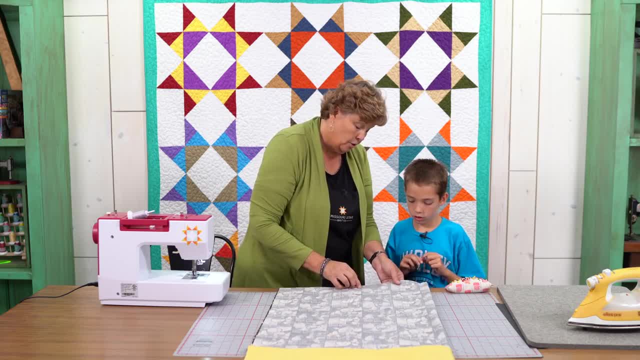 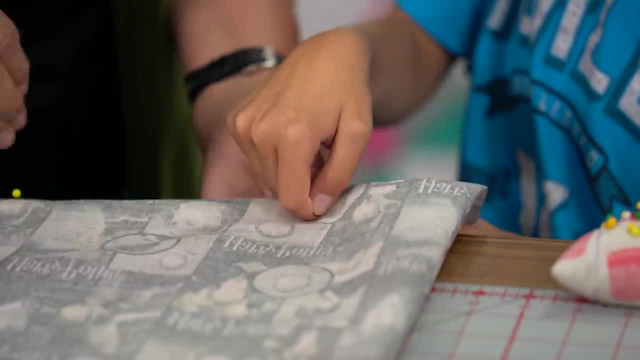 is super personal, because some people love to pin and some people aren't. They don't do a lot of pinning, So and I think that might have a little bit to do with experience as well. Alright, now I think we can take this guy out. 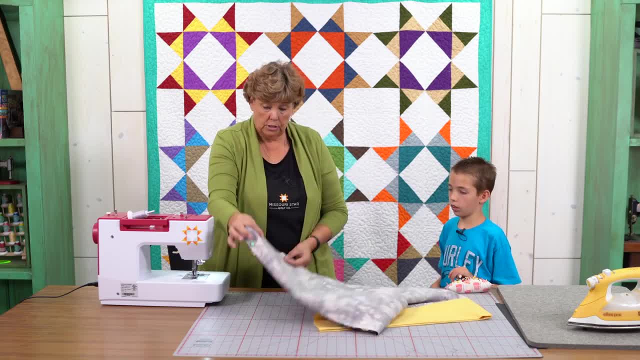 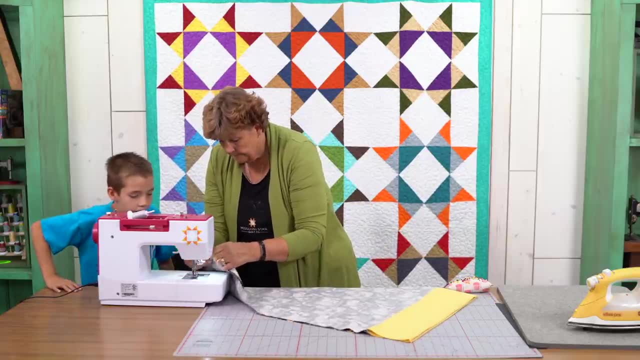 because we're going to start sewing right there, And we'll just sew right down this edge like this: Ok, Is your chair close enough? Shall we scoot you in a little bit Here. There we go. Can you reach that petal? 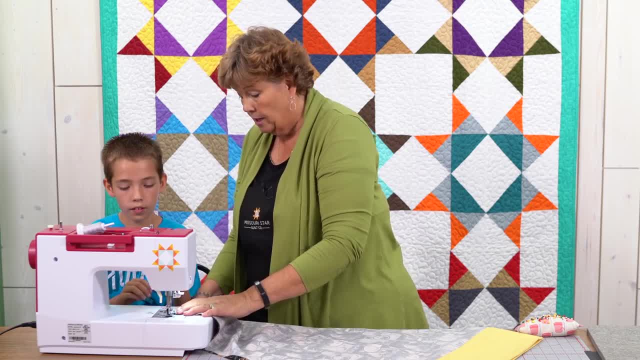 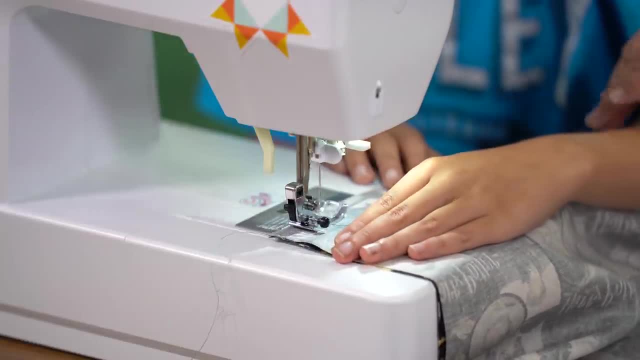 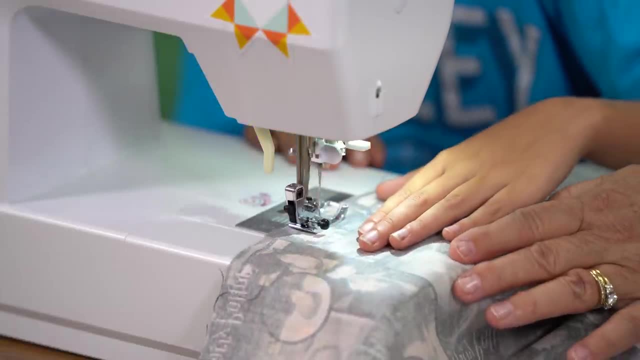 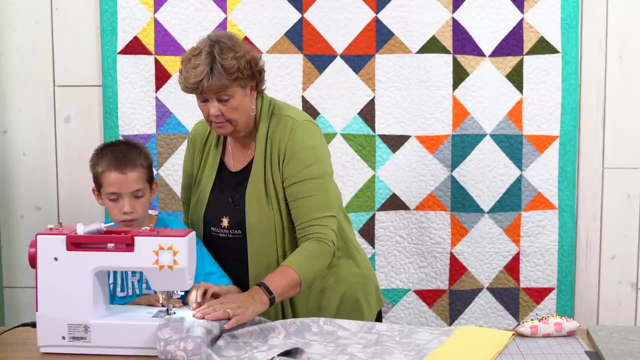 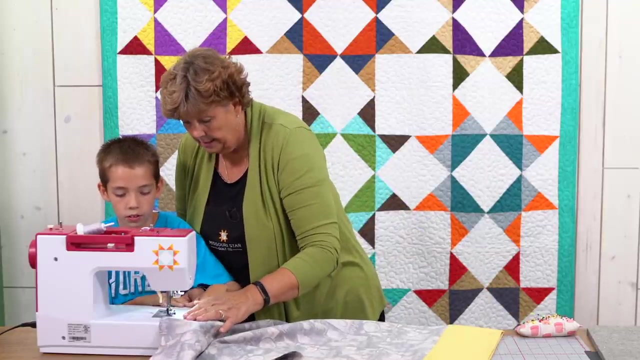 All right, Tell me if you think you can go faster. I think I could go faster. Do you think you can? You got both hands on there, Uh huh. Alright, you ready to watch it? Keep it out at the edge. Alright, I'm going to turn. 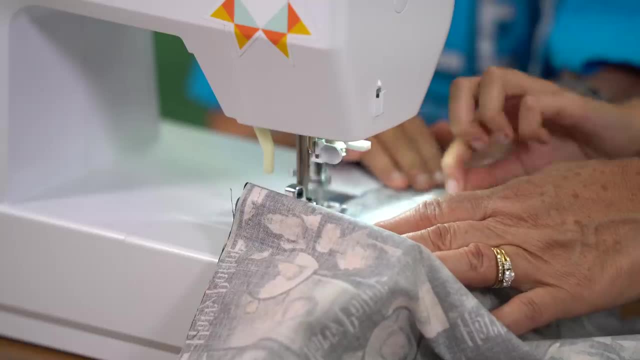 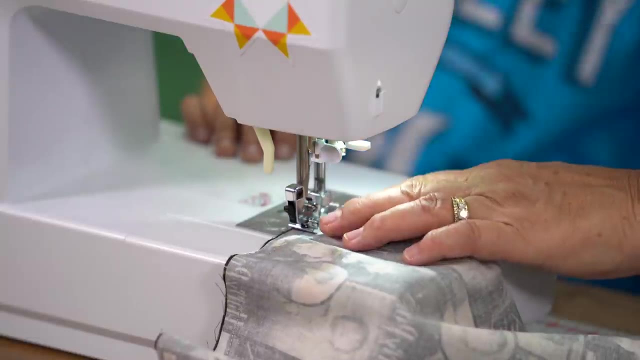 it up just a little bit. Woo, baby, Tell me if you think it's too fast, Come on. Come on, You're doing good. Alright, now, right here, stop and let's back up right here. So we're going to back up. We have this little back up stitch And then this little button makes. 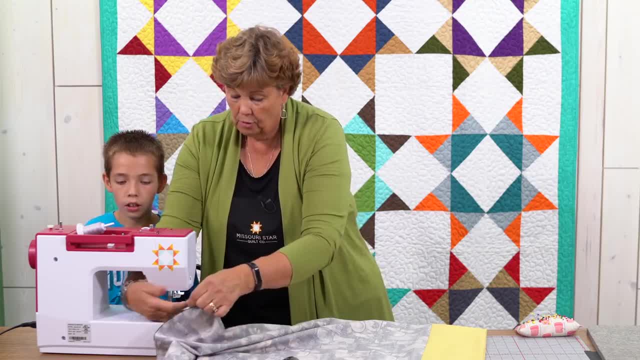 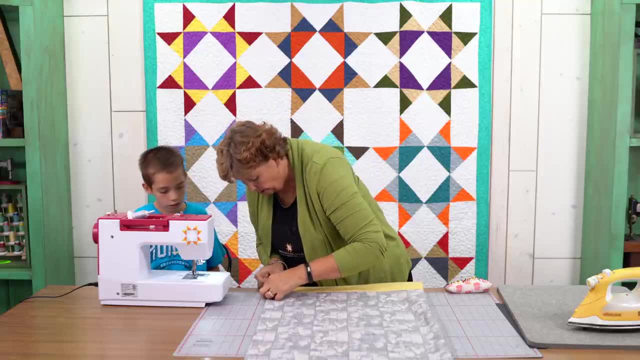 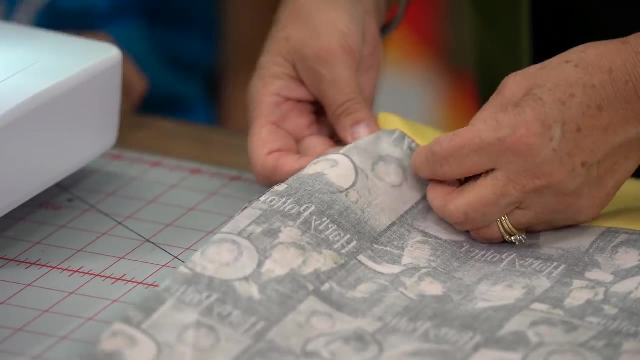 it go forward. There we go. Alright, now we're going to sew down the side, And when I sew down the side, I just like to make sure that these two pieces right here are matched exactly. ok, So I'm going to put a pin right there And then up here at the top. there it's. 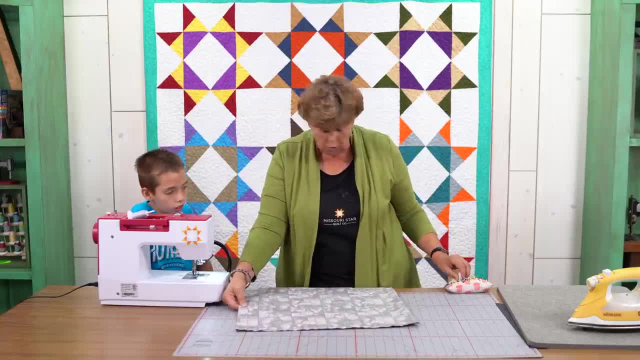 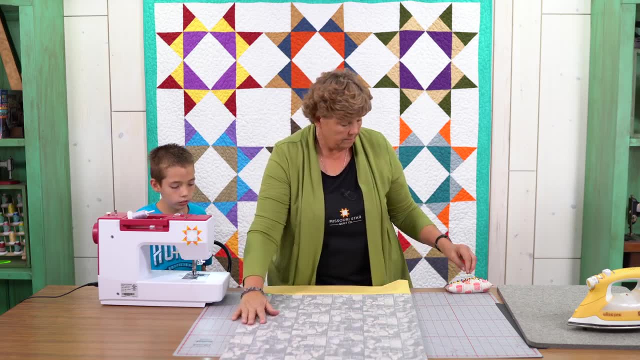 already sewn. So do you want to try no pins, or are you going to put a few, Maybe? like a few, Ok, How many do you think? Like three, Like four, Oh, four, ok, I love that you have an opinion. 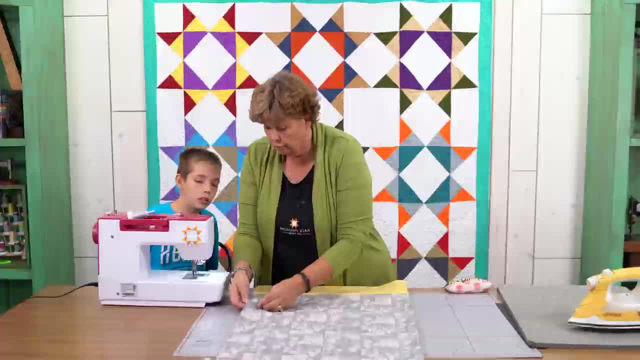 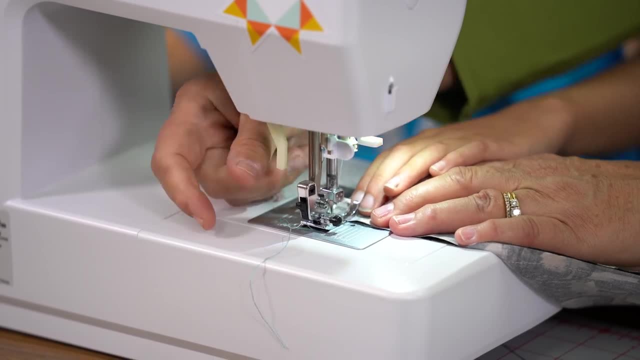 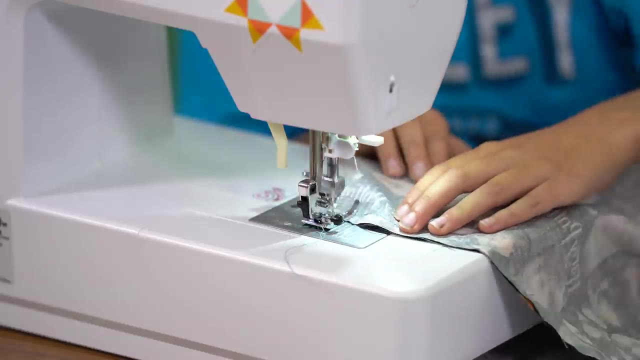 about your sewing pins? Alright, there's four right there. Alright, let's start here and go right down the side. We've got to lower our presser foot. Watch your fingers, Don't let them get too close to that needle- And I will try and hold this up so you can feed it through. Alright now. 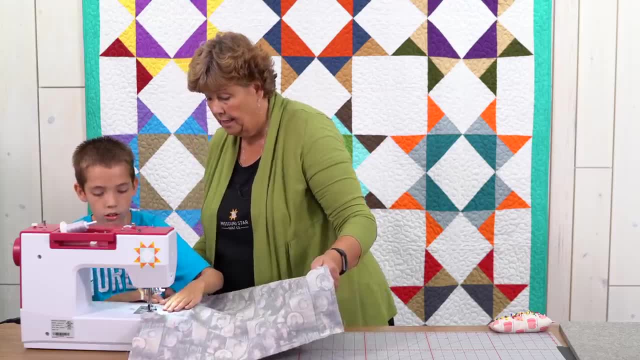 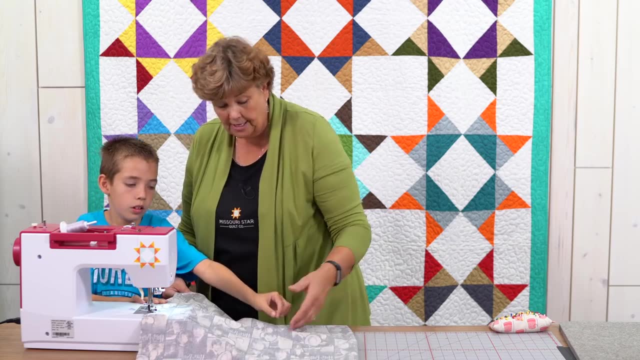 when you want to take a pin out. if you want to stop and let off the foot pedal, you can, And then it won't move. You won't have to take your hands off it while it's sewing because I like to keep my hands on Yep, just like that. Perfect. 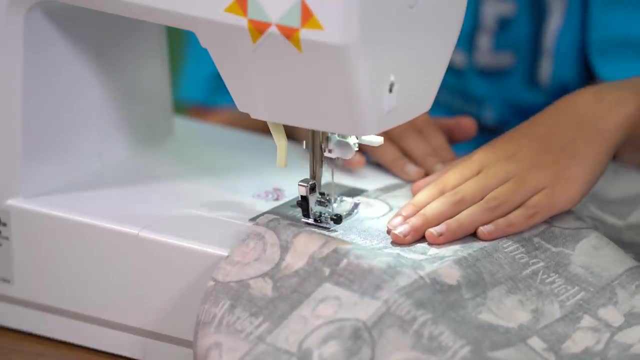 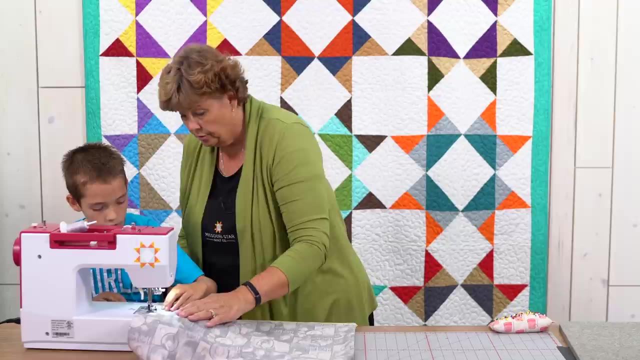 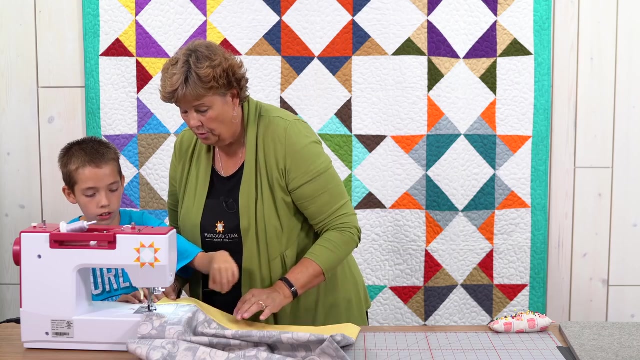 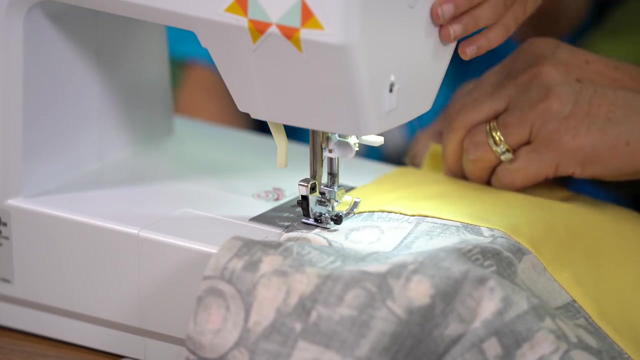 What do you think? Are you liking this? Uh huh, Alright, I've got a good job going over here. One more: Put that in the pin. cushion. Alright, stop, Alright. now we have a little bit where our seam is a little bit off right there, but we're going to keep sewing because 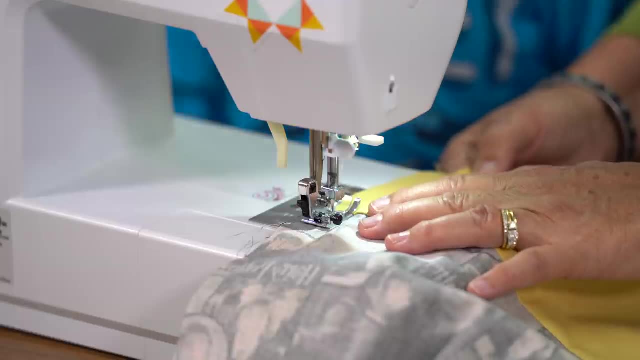 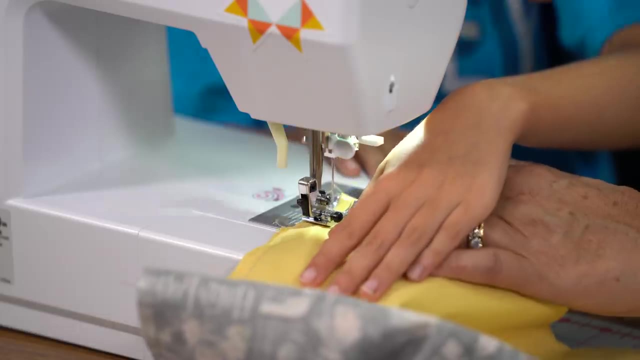 I know I'm going to catch it, So let's go. So let's just go ahead and sew on right there. Alright, now put your hands back up and we're almost to the end, And let's- let's sew backwards now for a little bit. 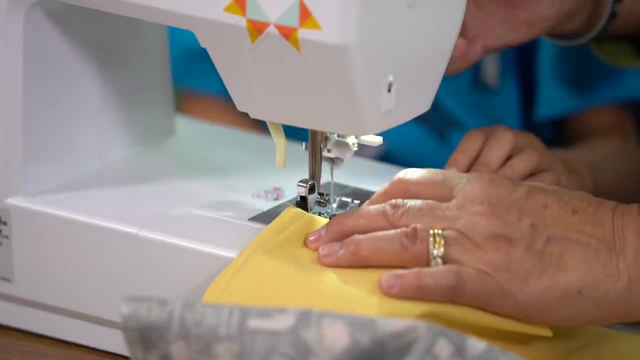 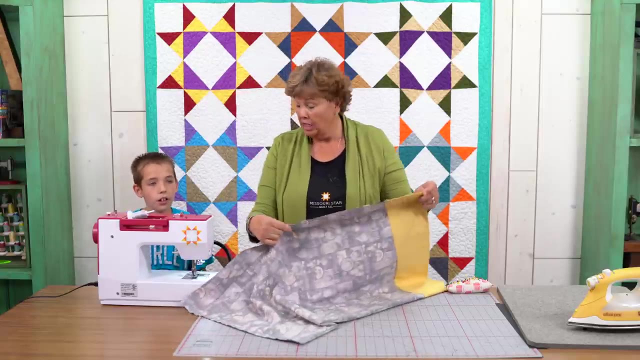 And then we'll sew forward And then backwards. Oh and then stop. Whew, Those button things. I don't love button sewing, but some people love it. They love that their sewing machine has a button you can push and it will just go. You don't even need the feet, Alright, 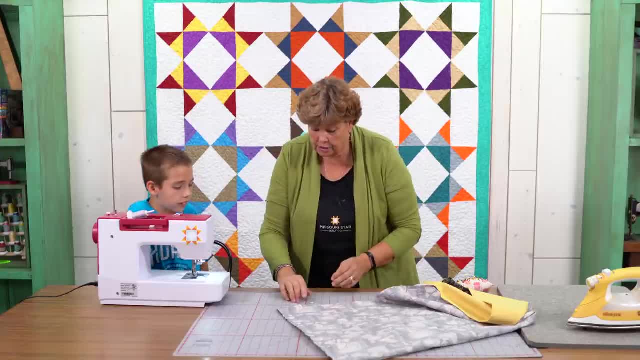 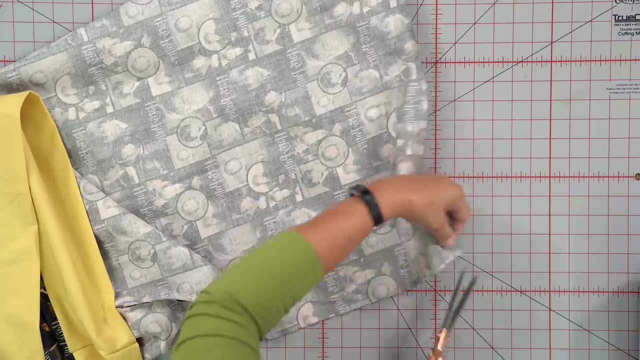 are you ready to turn this inside out? Yes, I'm ready. Are you ready to turn this inside out? Yes, One of the things I like to do- and this is just a little finishing tip, you don't have to do this, but I like to do it- is on these corners, right here. I like to trim them. 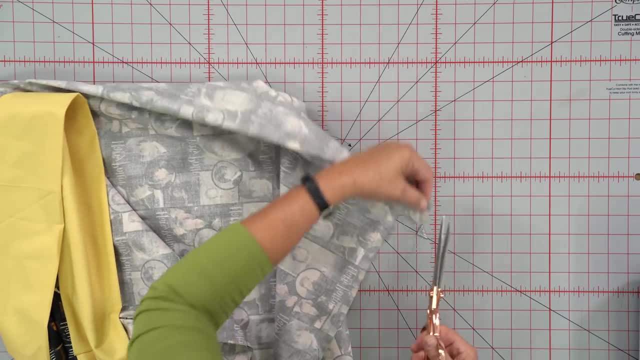 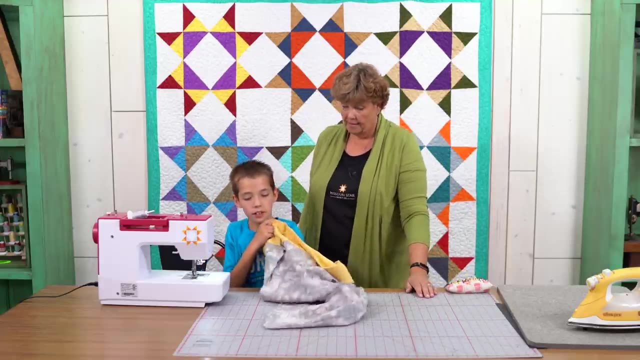 off, just like this, And then this corner too, so that the corner is crisper. It makes it turn nicer. Alright, you ready to turn that right side out? Uh huh, Grab all the way up there and grab that. There you go. Look at this, you guys, This. 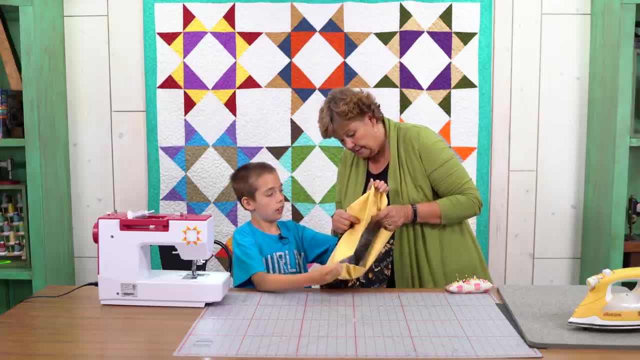 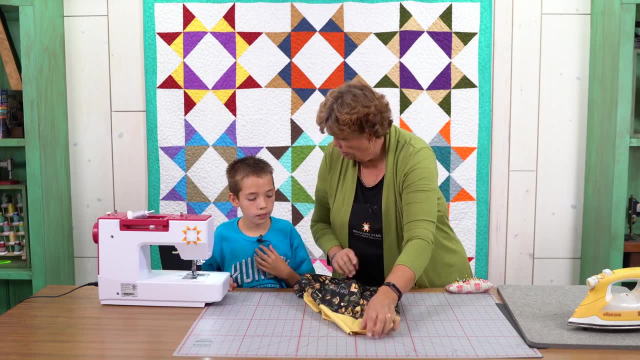 is looking really cool. Wait, let's check and see if we match this up. You know what? That's pretty dang good right there. Alright, look at this. You did pretty good. Actually, it was me pinning, So it's pretty good right there. Just the hair off, but nobody's going. 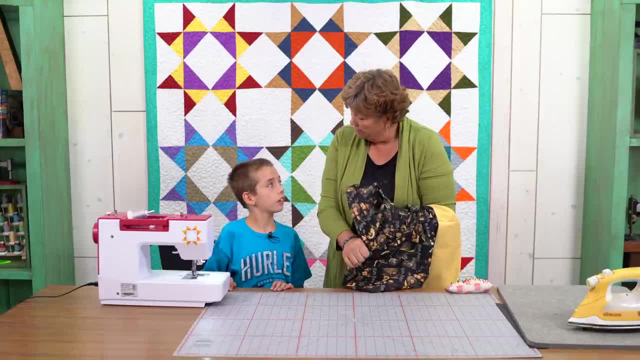 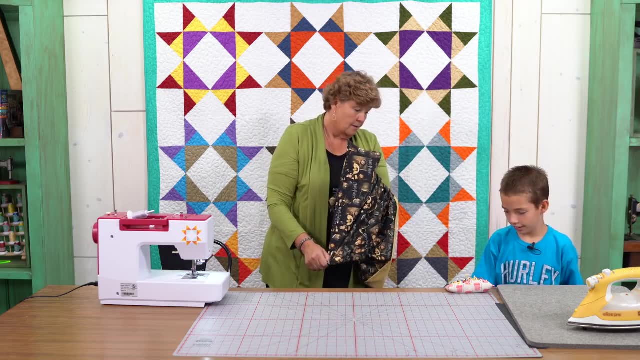 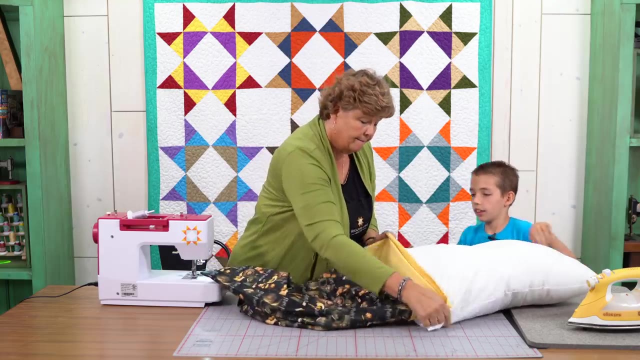 to die over it. are they Finished is better than perfect, isn't it? Uh huh. Alright, do you have a pillow for this? Uh huh, I think there's one somewhere down here. He's got it right under there. Alright, let's put it in here and see how it works. 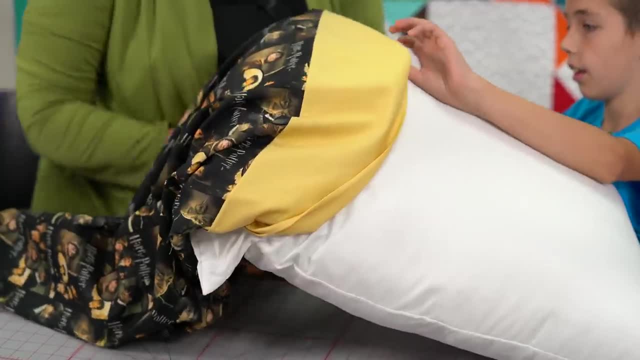 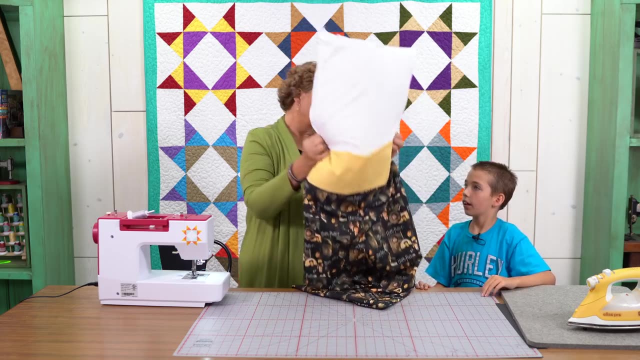 Do you get to mix? Do you get to change your pillows at home? No, not really. No, not really. Well, once your mom sees this video and she sees that you actually know how to change pillows, guess what's going to happen. What? 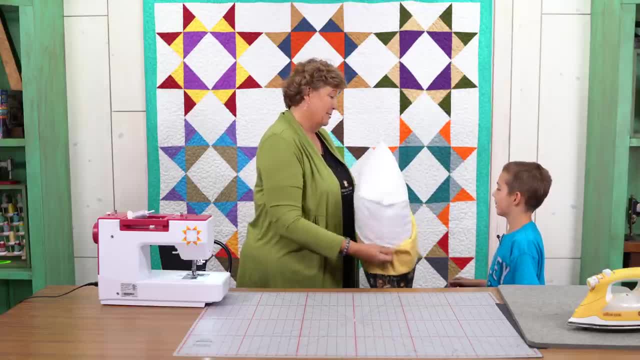 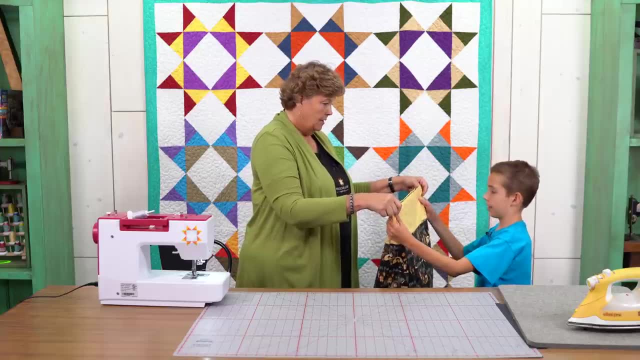 You're going to be doing all the pillows. Actually, I'm doing this mostly, aren't I? Uh huh, I just like to shake them like that. It goes all the way down and guess what? We made a pillowcase. We made a pillowcase. Look at that. 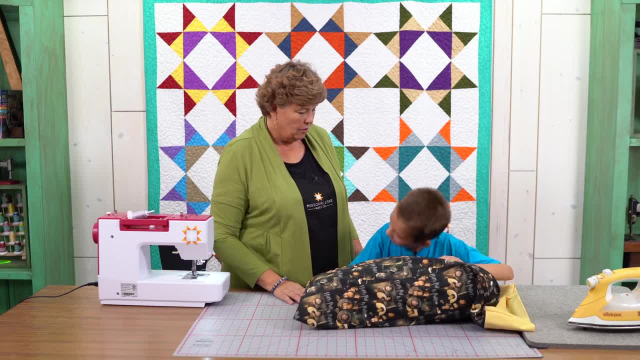 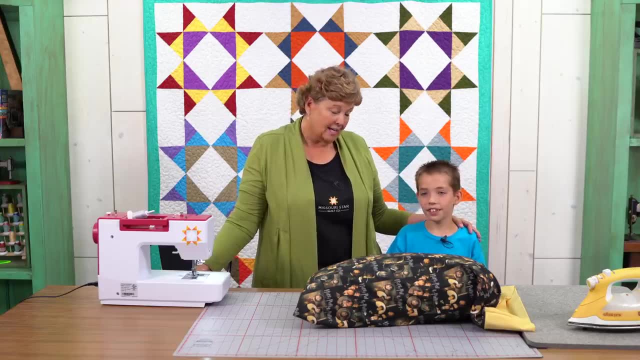 Is it soft? It's soft enough for you. You want to try your head on there and see if it works? Yes, it is. I think you're going to have some good sleeps while you're here visiting us in Missouri. So have you watched any of my videos? 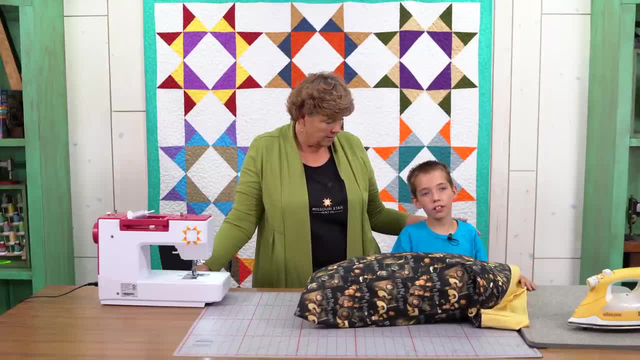 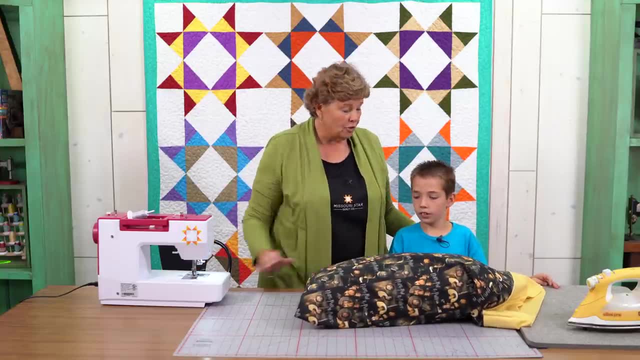 No, Do you know how they end? No, Well, how I say them is I say so. today we made a pillowcase and we hope you enjoyed watching this pillowcase tutorial from the Missouri Star Quilt Company. Can you say that? Uh huh? 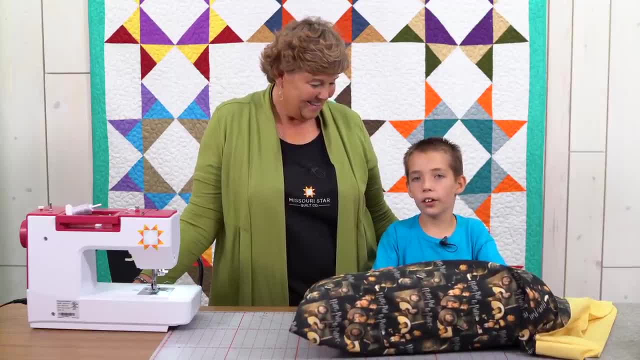 Alright, I hope you enjoyed the pillowcase tutorial from the Missouri Star Quilt Company- Perfect. Thanks everybody for joining us.